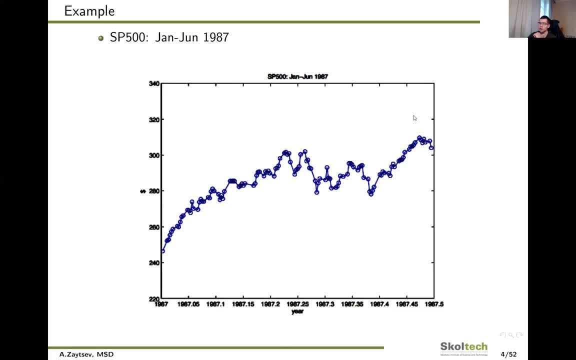 It has a strange structure and a lot of peculiarities And also it's particularly obvious that we need to work with this data to extract some value of it. For example, we can try to predict this data. We can also estimate on the confidence intervals for any part of this data. 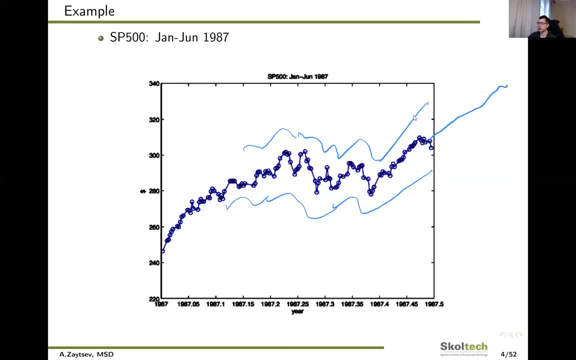 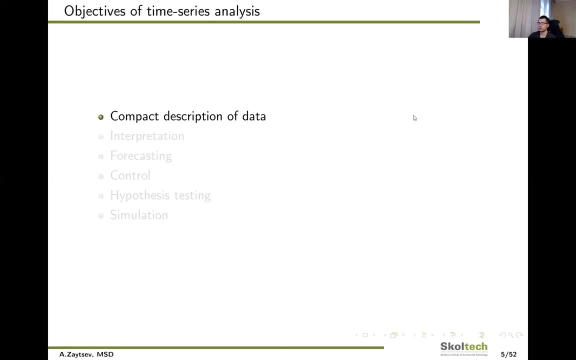 Or we can try to extract some embeddings of the data as a whole, And as this time-series is pretty simple, we don't have much here to discuss. We can try to model explicitly what we want from this particular time-series, And we have a lot of points to cover here. 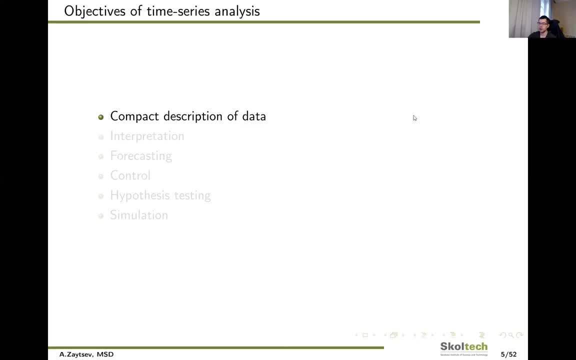 The first one is complex description of the data. In this case, we want to, for example, go from this like a lot of measurements we have in the data to like maybe one or two coefficients. that represents the main properties of it, And so we can compare one time-series with another time-series. 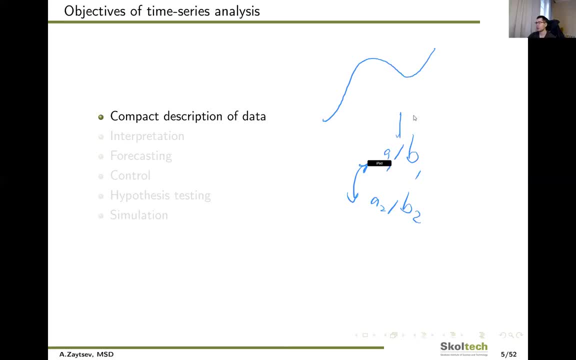 and say what's if one is better than the other. or we can say what is the closest time-series and what is the closest station to what we have right now when we are talking about some market. Also, as long as we can provide consistent models for time-series modeling, 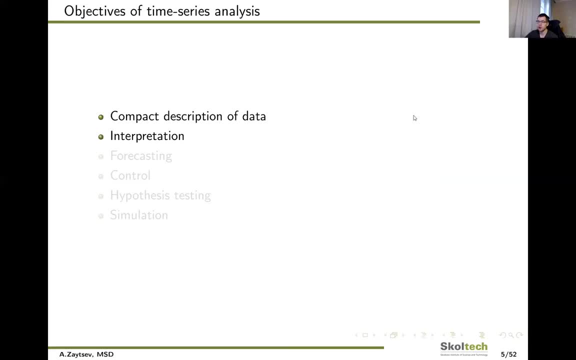 we can try to create some interpretation for the results, like we obtained, for example, for these coefficients we extract from the data. We can say that right now it works good, but later it works not that good, and so on From the problems that are related to the description. 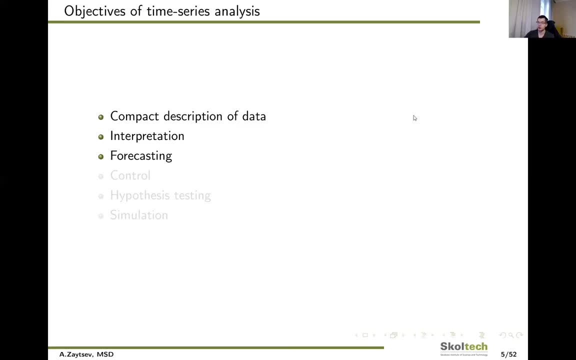 of what's going on with time-series. we can try to project what we know to the future and try, for example, solve a forecasting problem. In this case, we have some time-series, for example, and we want to continue it in the future. 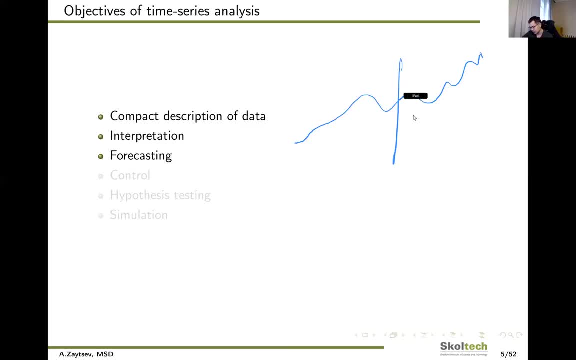 and this prediction should be accurate. so if you have like true time-series, it should be close to what we have as our prediction After forecasting. so we can say that these two guys is about like descriptive modeling. It's kind of not yet prescriptive. 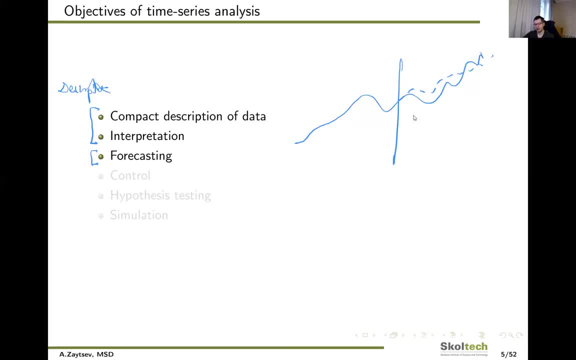 but it describes on how. Okay, Like predictive modeling, I would like to say here: Later we can try to do prescriptive modeling, So we can try to identify what we should change to make the behavior of a particular time-series better. 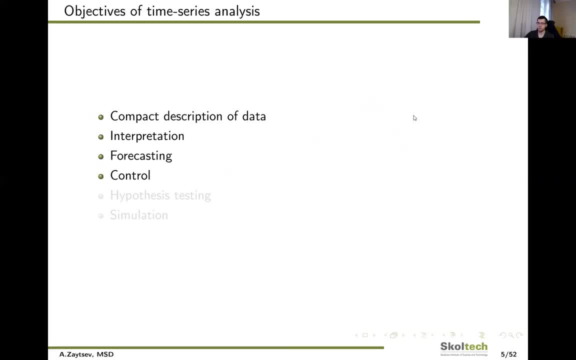 And in this case we are like: encounter this control theory and this control problems. but if we are talking about machine learning, for sure we don't have much to worry about, I suppose, in most cases, and the control approaches are pretty simple for most cases. 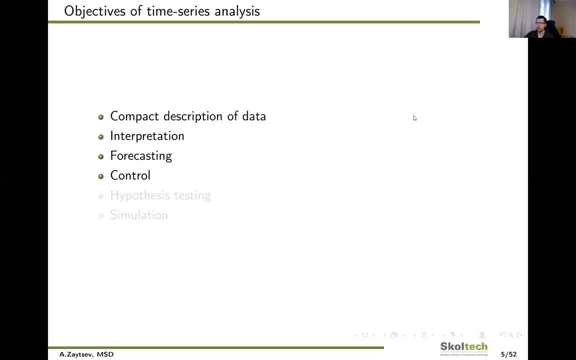 but for sure, we can apply this wide range of tools available from control theory to make these results even better in some cases, especially if we have this like theoretically deep understanding of what's going on in our time-series Now, last but not the least, 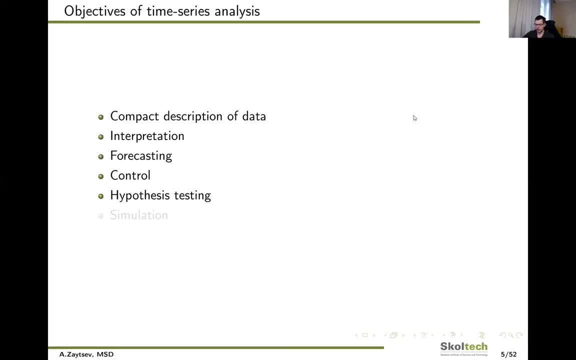 we can try to check something about this data- Maybe it's related somehow to the first point or to the second point- and we test if the time-series is stationary or what it will be in one month and if this situation is similar to what we had before. 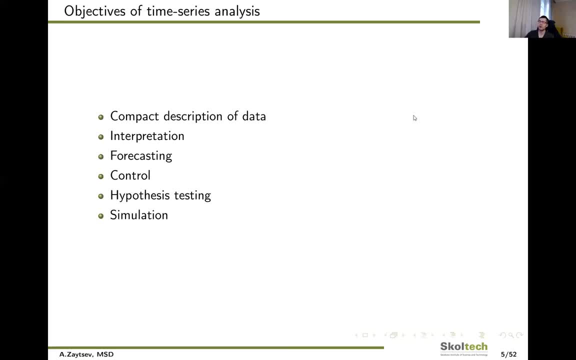 And also, as we have these fully controlled models, we can try to run this simulation and try to write different scenarios and describe what's going on and what will go from this particular moment in the future. For example, we can change one control parameter. 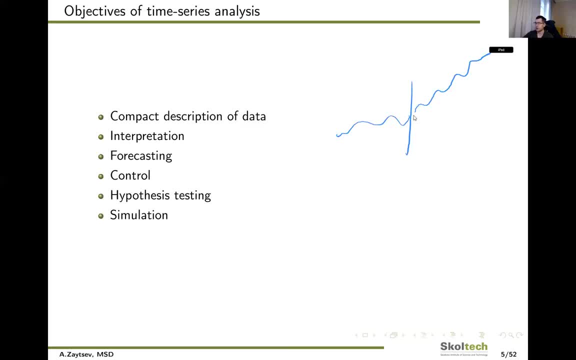 and say that it's quite probable that we will have time-series like this. This is like the first scenario And also we can try different scenario for different set of control variables or different station about what we don't have right now, And this is what we also can do. 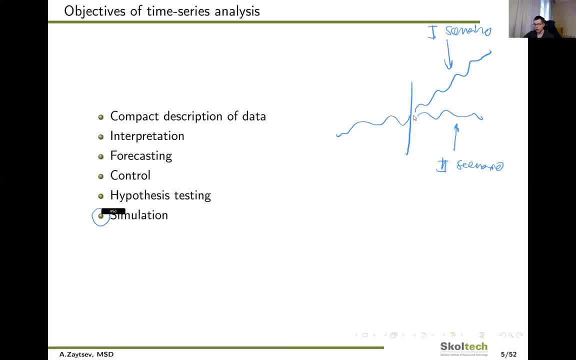 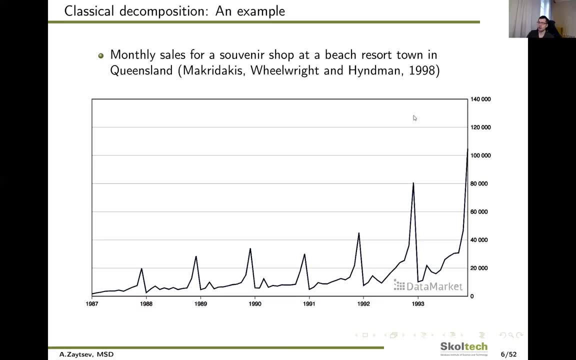 with this simulation part of objectives for time-series analysis. Let's try to start with some decomposition and with some classic model on what time-series is about. A good example, and a pretty common example, of time-series is this: data on monthly sales for a small shop at a small town in Queensland. 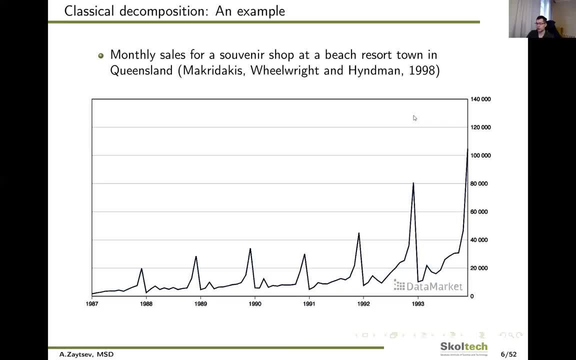 We can see that this data is collected more than 20 hours ago. From what we can see, we can identify these peculiarities of the data that we will later reflect as the model structure. We say that we have right now these peaks, These peaks, all are about the end of the year. 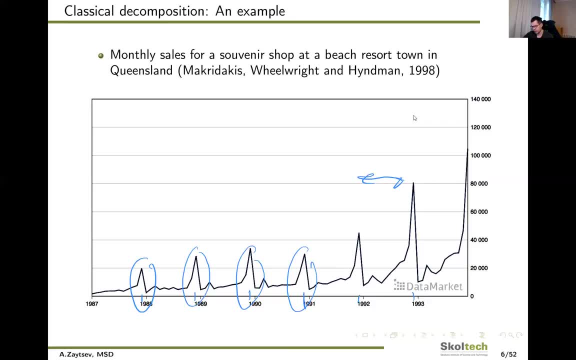 So we can say that we have some periodicity, and the period for this data is about 20 months. Also, in addition to the periodicity, we have an increasing trend. We can say that each year this peak is slightly larger than it was last year. 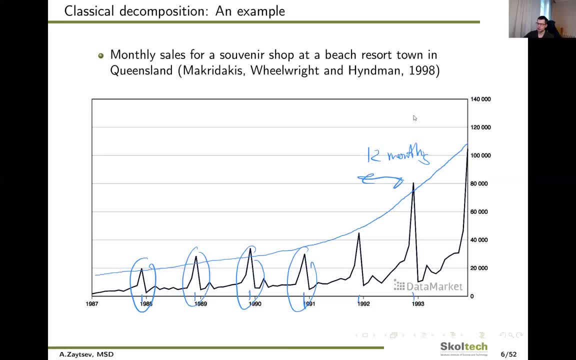 And it holds not only for the peak value in December but also for the general trend in the data we observe. So we can say that we have increase in sales and this small shop is very successful. But this is what we should include in our model assumption. 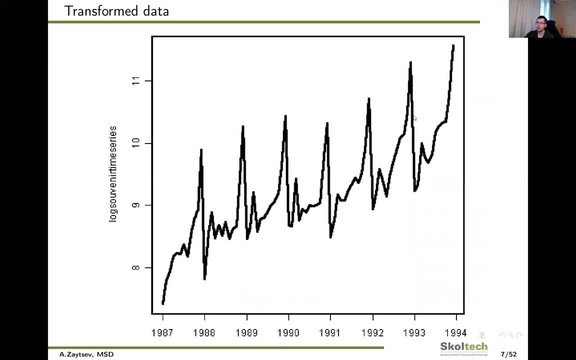 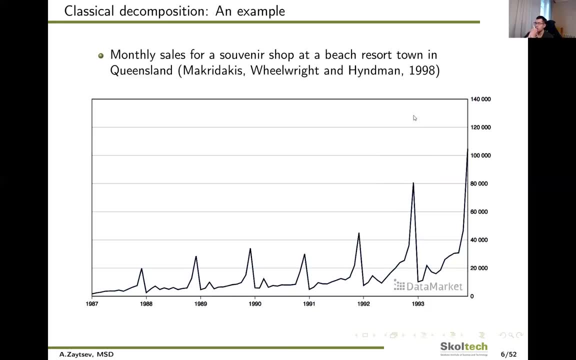 for forecasting, for example, of the sales, to be accurate. But what also we can see, and what complicates our time series analysis, is that it has different scales during different years. We say that in the beginning it's like below 20,000. 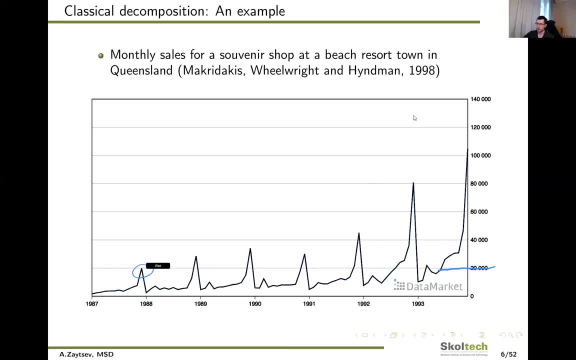 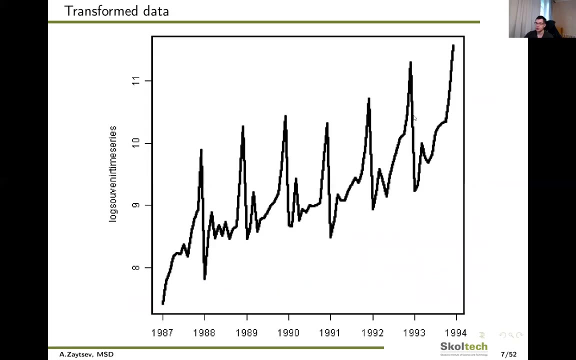 and even maximum value is below this particular value. But as we observe more and more data, we have increased, like about five times. So okay, to make the analysis proper, we normalize the data And after normalization we have some stresses. 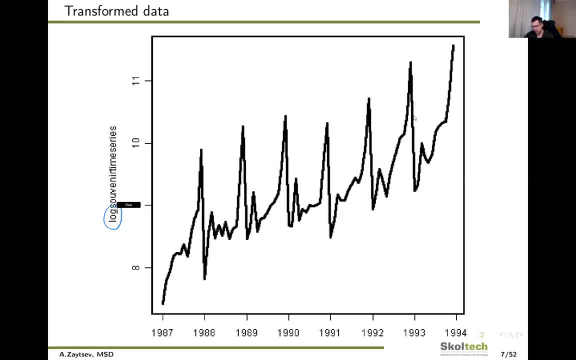 In particular, we use log transformation, So we take a logarithm for each value we observe in the data. It's a legitimate operation because for each value it is positive. That's because it's amount of sales and this amount are always greater than zero. 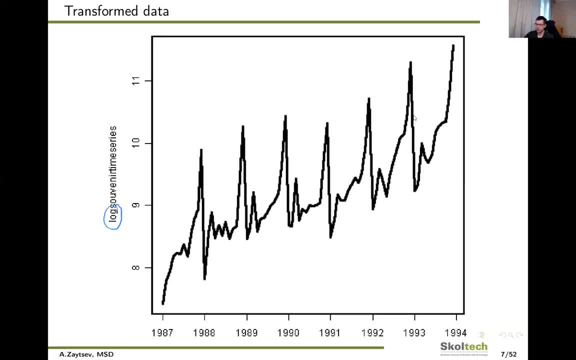 So after the transformation, we can transform data like this. It looks like more uniform and we don't have this sharp increase. We still observe the trend is increasing, but we are still happy that it's not like five times. It's also only linear scale changes. 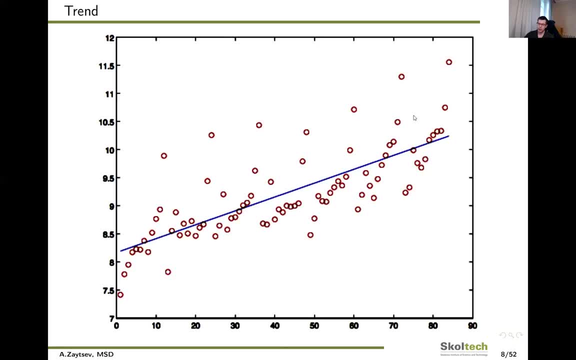 Okay, we normalize the data, make it look more stationary, and we will talk later about what the stationarity is and why it's so important for this particular case. But now we want to try some model, And usually if we don't have much data, 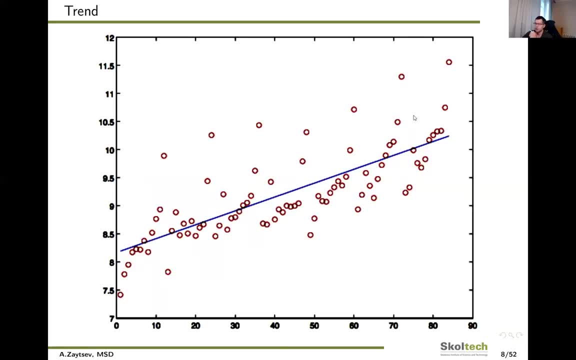 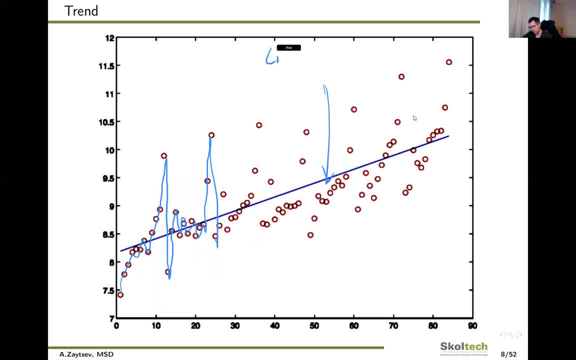 and we observe this blue curve that help us to identify what is the trend in the data And we observe it increases in general. And also we can, I hope in this case, justify that the coefficient for the linear regression as this angle on how big the increase is. 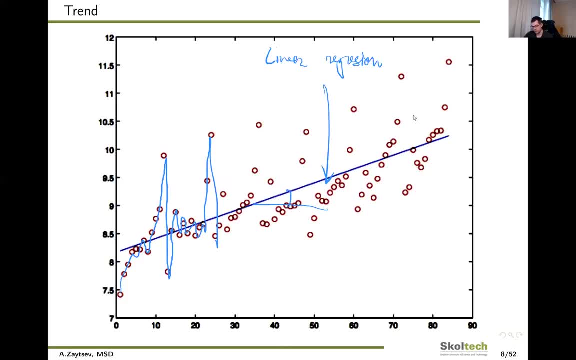 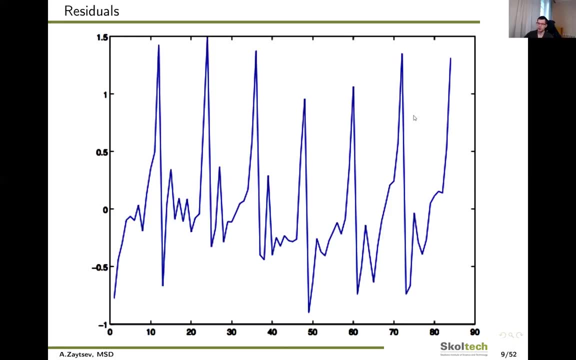 is significantly bigger than zero And it's even statistically significantly bigger than zero. Also, after application of these two operations- normalization and trend extraction- we can try to analyze what's left, What we can't explain, with this quite smart and reasonable model. 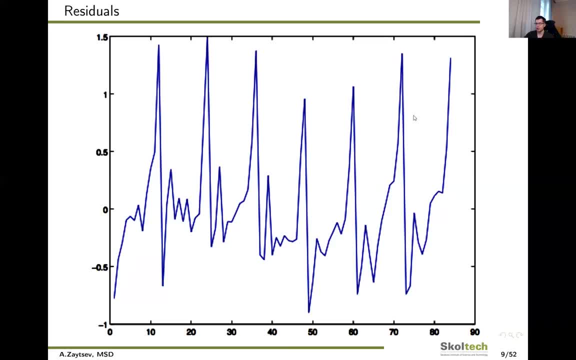 In particular, we can look at the residuals. In this case, this is the difference between the trend value we predict- Okay, let's say it by hat for time t- and the true value we observe from our data. We can use an absolute. 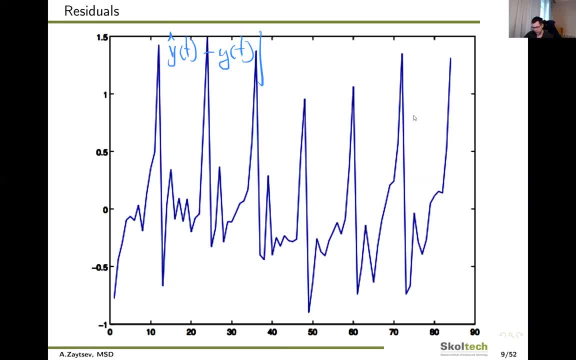 value of this difference, or we can still see only the okay, not absolute- values, And so we can observe here, for example, negative values, And so we can use that value to help us to understand that sometimes we don't estimate this trend quite well. 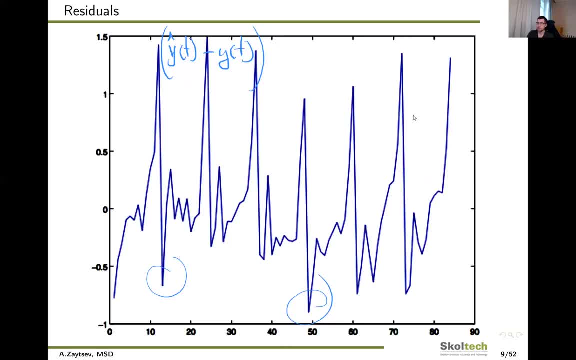 in terms of both increase and decrease, And we can specifically analyze here. why do we observe such behavior? In this case, it's pretty obvious. We have these peaks related to the end of the year, And we have these peaks, but of the other type. 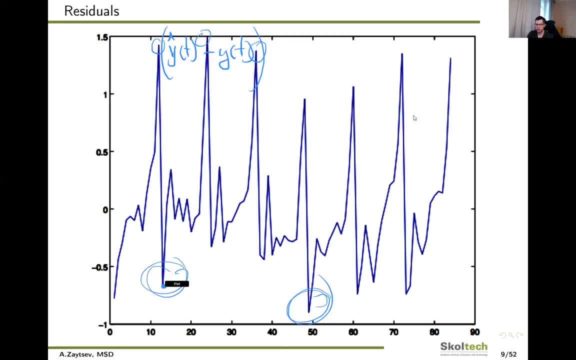 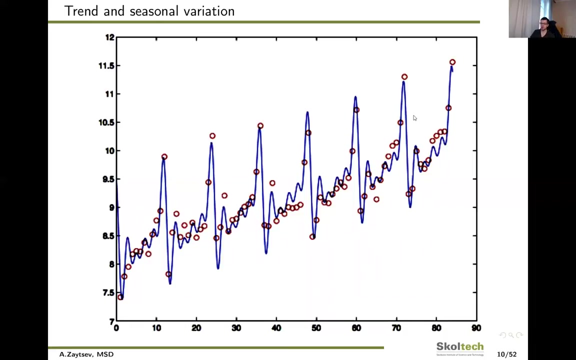 when we look at the lower part, in january i suppose no one buys these groceries or whatever this shop sales, because maybe no one is traveling in january and or they spent all of the money devoted to seven years or last months. but whatever, uh, we can try to adjust the model to take into account that we have this residuals. 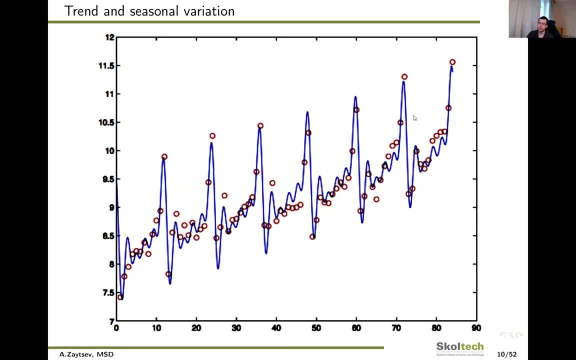 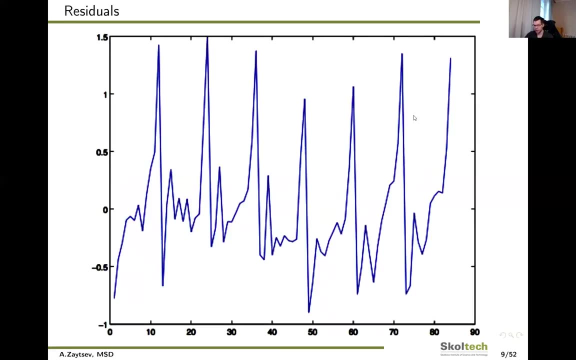 and we can try to explain it in ways common to time series data models. for this particular case, we say that we want to identify seasonal variation and include seasonality in the data. so if you look at the previous guide, we can say that we can repeat the same pattern each year. 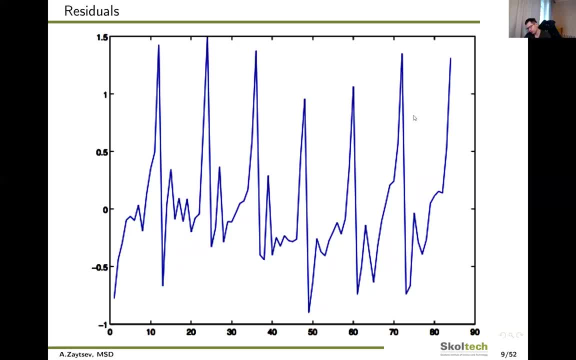 after year, something like this. so it has a similar up and down values and also it has kind of few parameters because we don't need to model each data point explicitly. we model only one period that we assume is presented in the data. so after adding of this periodic 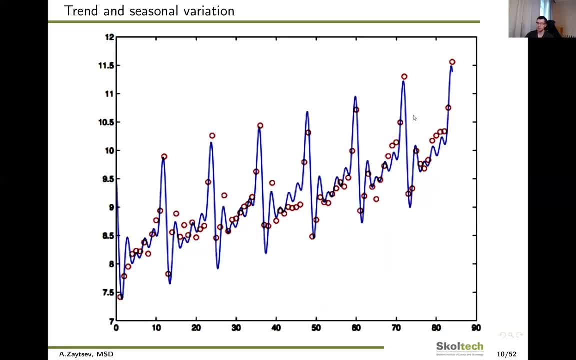 seasonal variation, this periodicity to the data, to the trend. we have something like this and, as we can see, it's pretty nice, much nicer than we have only with a linear model or without any model at all, without scaling and so on. and we also see that all these steps of water, instead essential for this particular data. 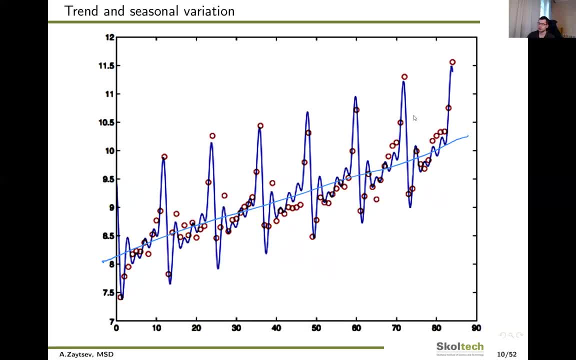 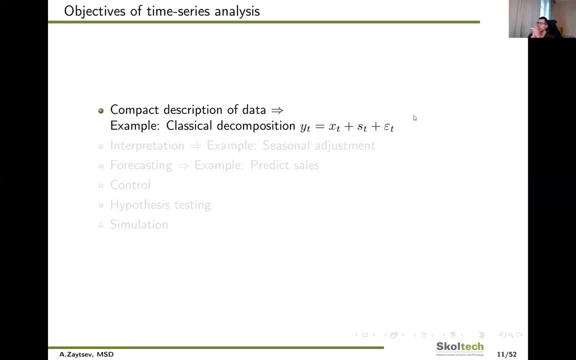 and it's quite common that we observe such behavior in many different time models. so let's see how we can apply this objectives to this particular problem of working with souvenir shop sales for about 10 years. let's say as a start that we have a decomposition of the data to a number of components. 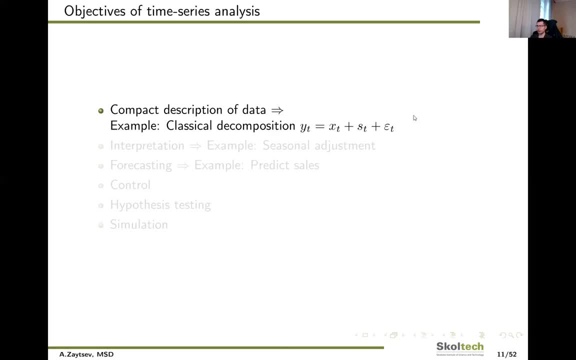 here we introduce three components, two components we talked about explicitly, like trend x, seasonality s and noise we haven't talked yet. also pretty obvious that it is presented and it can be interpreted as noise itself or is something that we don't have enough knowledge about. so after the representing of the data in this way, we can try to interpret what we have. 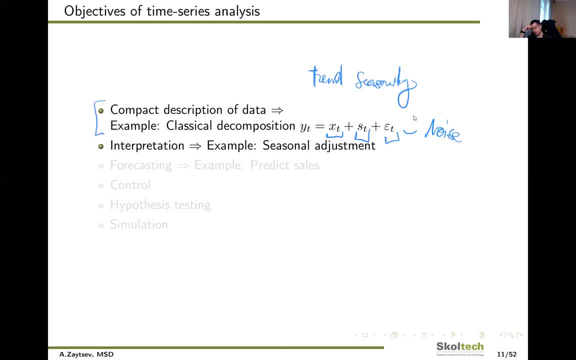 for example, we can say that we have seasonal adjustment here and we need to enforce it, and we can even try to base our decisions on what we have, or somehow measure some macroeconomic indexes on the base, on the sales in this small shop as a shore or somewhere in united states or maybe not even. 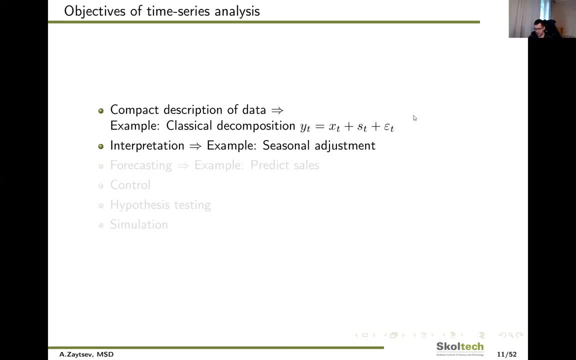 united states. we can go on and try to do some predictive analytics. for example, we can try to predict sales next year, so we can plan logistics, we can plan how much order should we do, and so on, and so on, and so on. in addition to this, we can try to use all these guys. 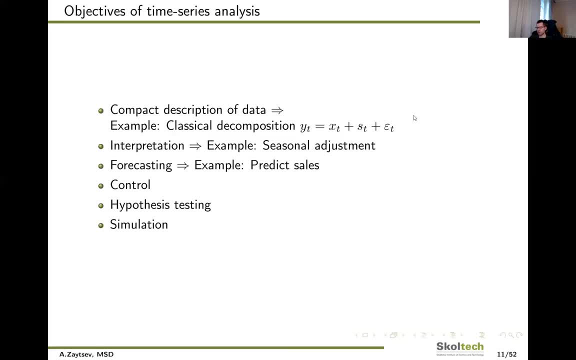 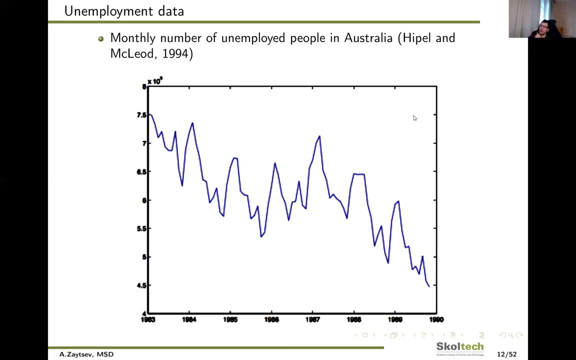 together. in this particular case maybe it's not that important, but for example for control, we can try to say that. or maybe we should hire another guy here and we can assume that we will have more sales if we hire additional personnel to help this shop and so on. let's also check on another popular 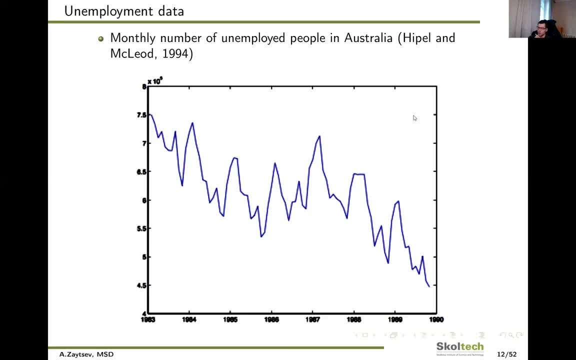 dataset. it's managing number of unemployed people in a very distant island and we can see that it also have some peculiarities we later explore. for example, we can try to again see the trend, maybe some periodicity here. who knows if this speaks article distance or not. we can check it. 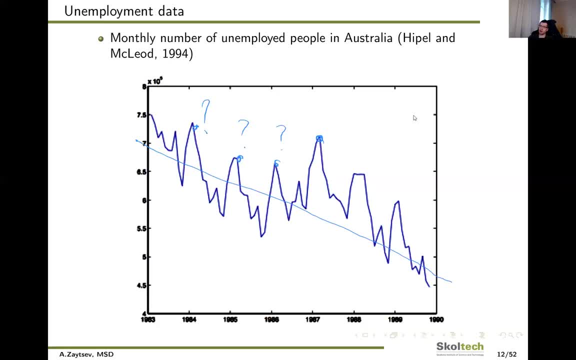 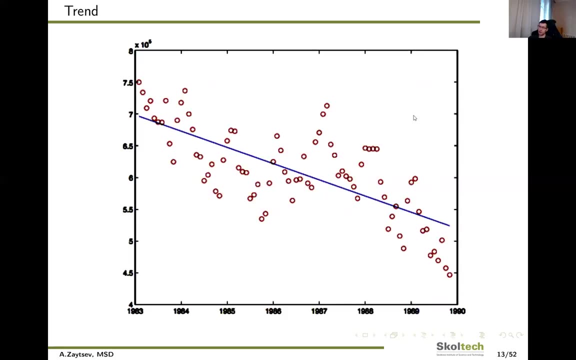 is in some simple statistical tools, and also also we. okay, we can try to have some additional components if you need them, and let's see what we can do about this particular time series. at first, we observe the trend and trend is pretty easy to grasp. here and again we see that we don't even need this long log. 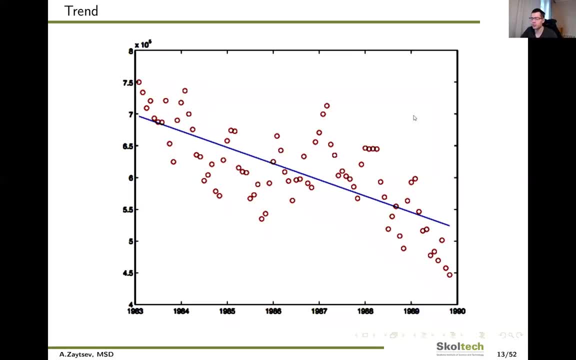 transformation, because the variable, this unemployment number of unemployment people- is quite similar, because, okay, I think that the total number of people is similar, that the central bank regulizes the interest rate for other banks, so we don't have different changes in unemployment and so on, but we still have some microeconomics that leads to the decreasing of the number. 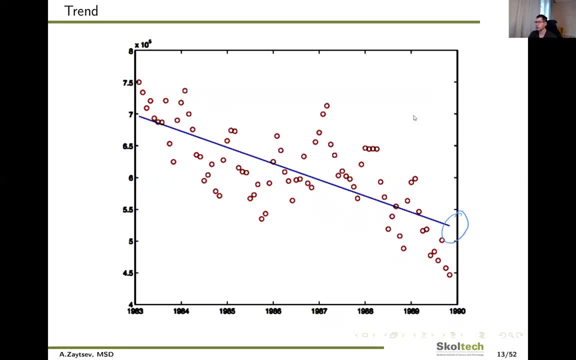 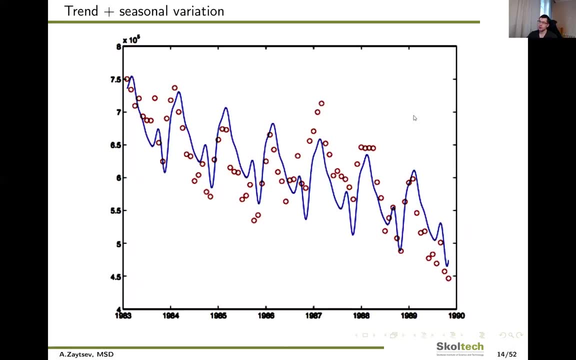 of unemployed people for this particular data and for this particular country, and so we start with modeling the data with a linear pattern. okay, again, we can try to adjust some periodical component of the time series and, as you can see, it's also pretty easy to grasp and pretty easy to agree that we really have this one. 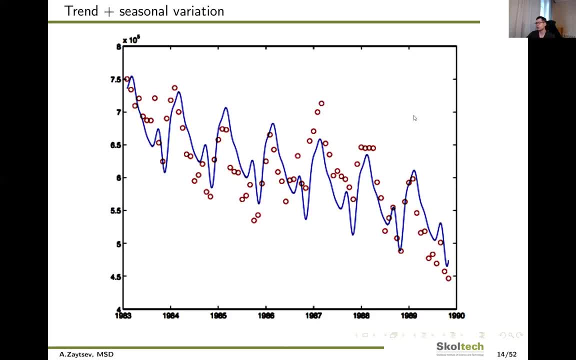 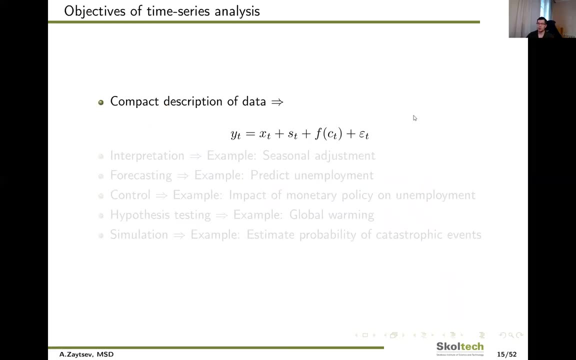 year periodicity, similar to what we had with this sales data, and in the end, we have something that similar to what we have before. also, when we are trying to match the objectives of them- serious analysis- with what we have and what we already done for this type of data. we observe three friends we already encountered during this lecture. 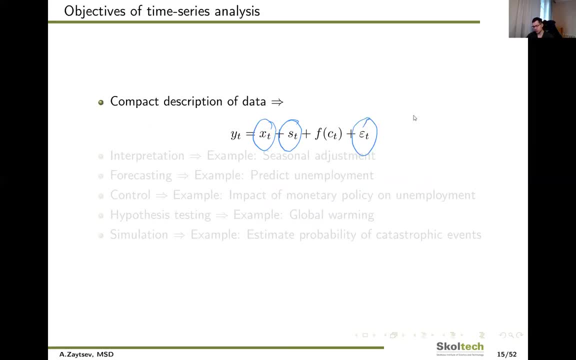 a trend- seasonality and noise- and one additional component that can be related to some latent variable that's not known, it's not presented in particular for this time series was pretty obvious: affects how big the unemployment rate is, for example. it can be some policy for this country or maybe even policies adapted worldwide, or it can be like a binary variable. 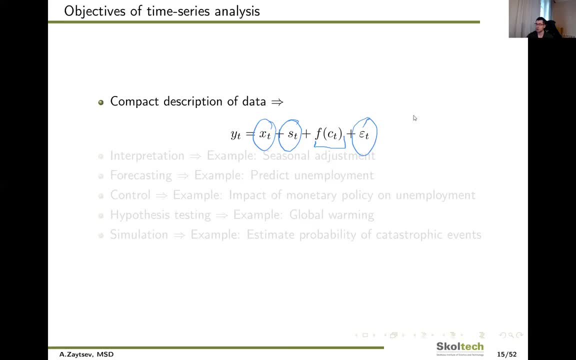 that reflects: do we have a pandemic of kovit 19 or not at this particular moment in this particular country? also, we can try to interpret this data. let's say that we have this variations related to seasons, uh, each time, so we can try to account for it and make either model more precise. 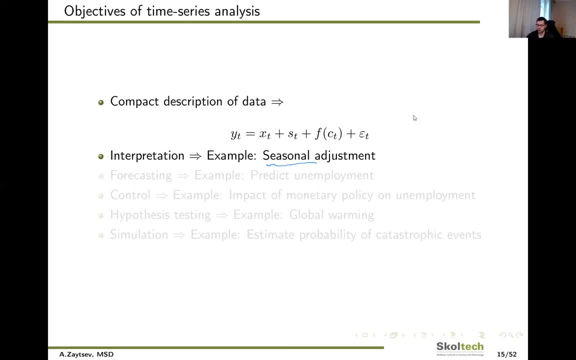 or maybe we can try to use it in a practical way to reduce unemployment or to correct the policies we have to make it more optimal with respect to the total success of the country. in addition to interpretation, we can for sure do a forecasting and predict unemployment rate in the future using the model we have right now. because 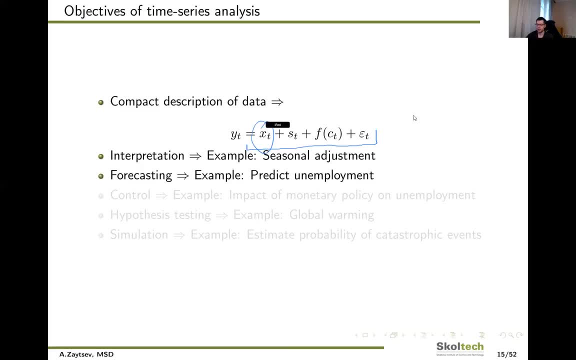 for trends, it's pretty easy to continue the trend as a linear function whatever long we want. for seasonal components, we also pretty easy can have something like what we had before and so on. and for this macroeconomic parameters, we also can try to model them in a way, and this part of 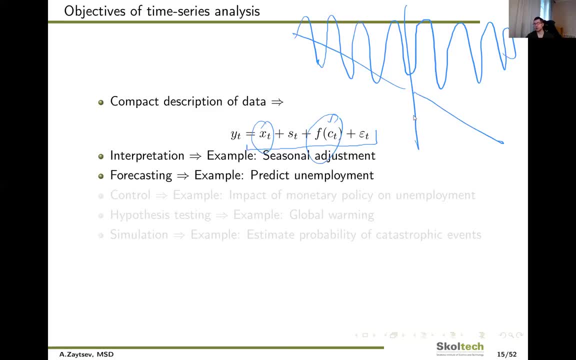 the model through our future observations and have, in the end, quite nice plot that reflects our interpretation about unemployment in the future, when we try to make it smarter and more useful for the population of the country and for the country itself. we can, for example, control the monetary policy and check how it affects 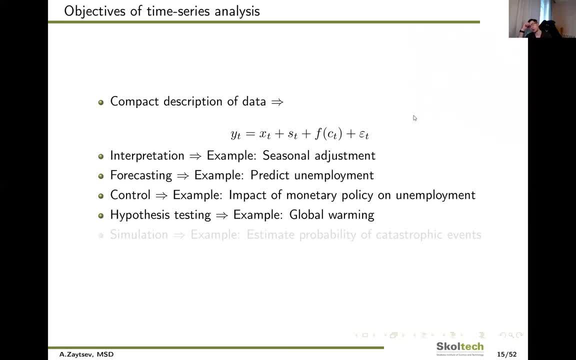 unemployment. also, we can do go in a different direction and try, for example, test: do they have a global warming or do global warming affects unemployment rate in australia? okay, whatever. also, and we can try to identify some particular patterns related to catastrophic events and for this catastrophic events we can try to estimate probability for them on the base. 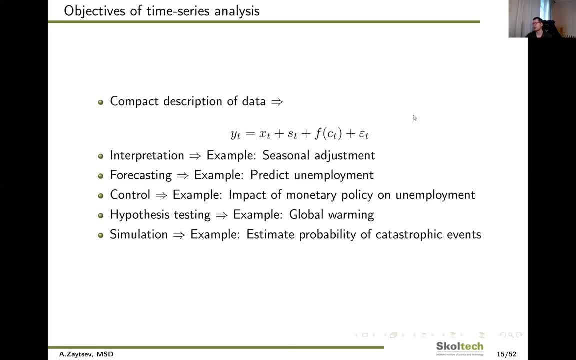 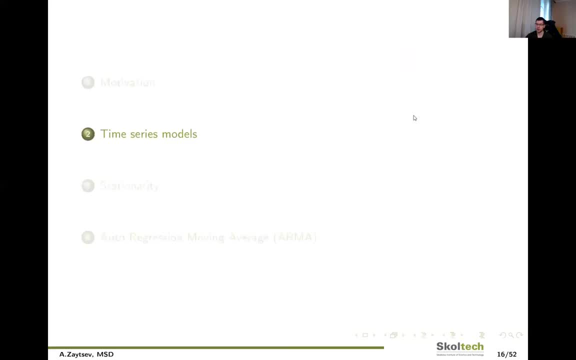 of the data and simulate maybe some scenarios and unemployment rates if the some events related to natural disaster happens. so we see that we can pretty easy link time series data to these particular points about the objectives of time series analysis and that in many cases it's pretty easy to spot something like this in the data and we often don't. 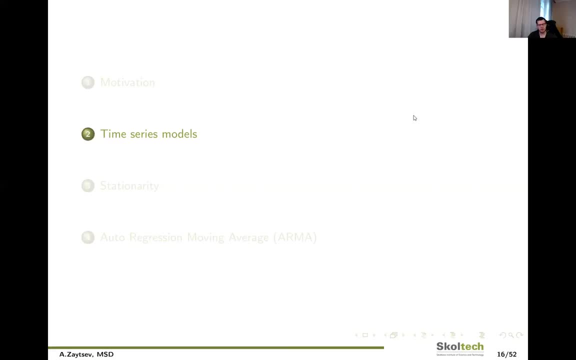 need quite complex models, so in this case it's enough to have this seasonality component and linear component, and this all we can do without neural networks. we don't need to learn the presentations if the data is simple enough or we have an expert that can provide some advice. 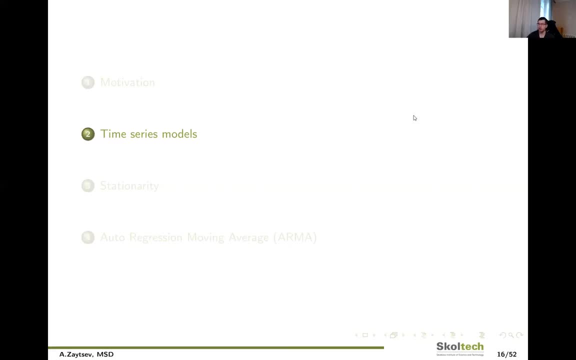 on. how can we select the model? okay, for sure with the help of a machine learning specialist, but let's try to form of this model. if we take what we can of course say this is a product of time series analysis, in the very beginning of the video we can analyze in more details what we can say about time series. 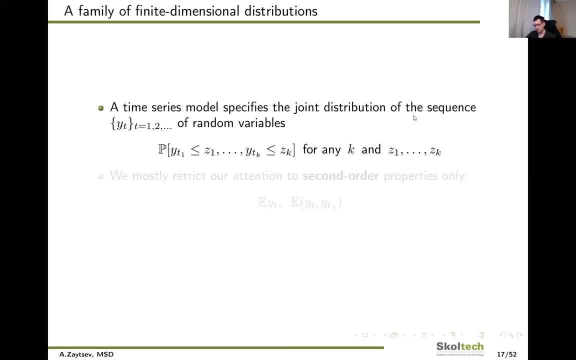 data, and so let's define it in the most general form in the very beginning. we can say was that if we observe some values- and yes, these values are random, because this time series and we have some noise, for example- we can model the distribution for them, each for the whole sequence here, so we have a sequence like this: 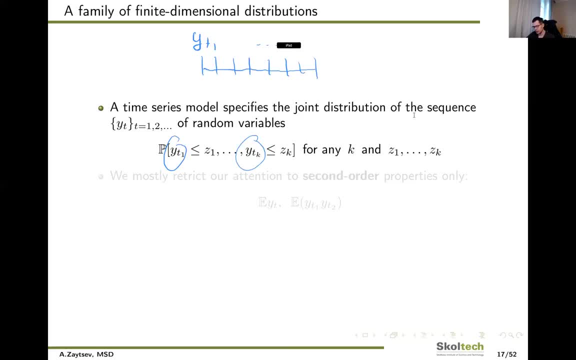 each time we observe y t1 up to y tk, and so we have a joint distribution for each and, for example, can identify a cumulative density function for this multi-dimensional random vector that is identified by this upper bounds, and so we have the probability for zk r2. 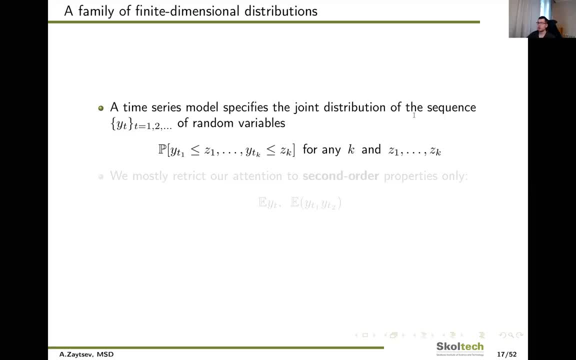 to get, okay, to get this particular vector. also, if you try to have a general model, in many cases it shouldn't be very useful because it would be too broad, too wide, not of any practical use, too many parameters and also we can't achieve goals specified before. for example, if you have two complex model, it's pretty hard to. 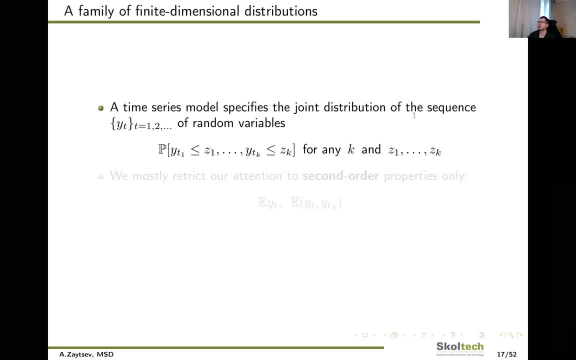 interpret this model, and so we are left with something we can interpret and okay, set story. so let's make it a bit more, a bit more happy, and try to restrict our attention to more useful in practice models and what we usually do in this case. we identify the mean value at each. 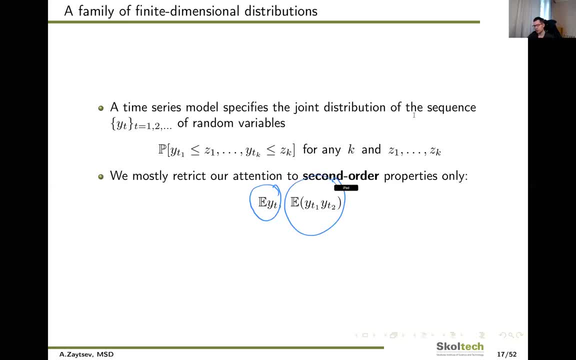 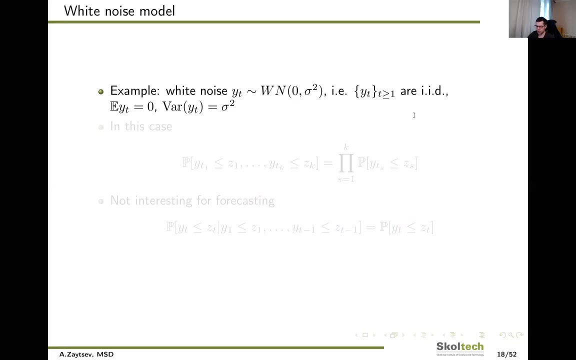 time step and we identify correlations of values between neighbor or far away observation here. so here is, for example, yt1, but here is a correlation between yt1 and yt2, and so let's start with specific this specification of yt1. so let's start with the distribution of the simplest possible model of white noise in this. 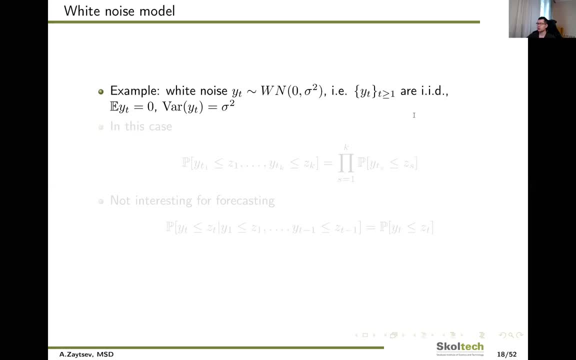 case, we assume that each value of y is independent and they can distribute it random variable, with some mean value and some variance. in this case, it's pretty easy to see that we have the decomposition of this probability to the product of probabilities related to the specific points. 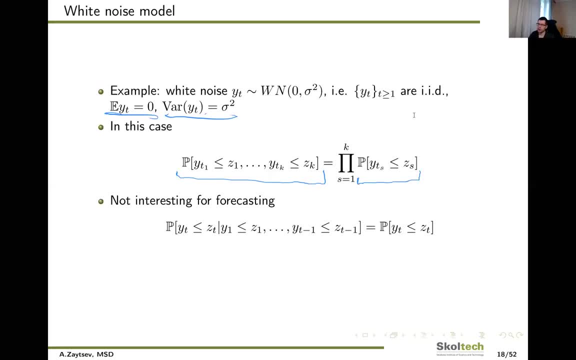 in time. we can say that we have independent random variables, so the joint distribution equals to the product of a one-dimensional distribution specific for each y here, and so you can say that this model is pretty simple and it's quite easy to imagine that we maximize this point with respect to some. 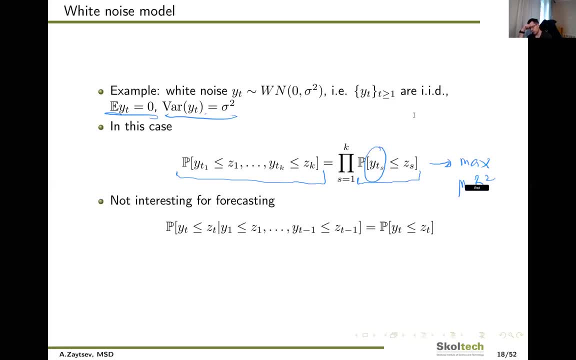 variance, for example, and some mean value if we use, if you are, some mean value instead of what we have before zero. but also we can say that this model is pretty useless for almost all use cases we can imagine. let's try to understand it for the case when we are forecasting something. 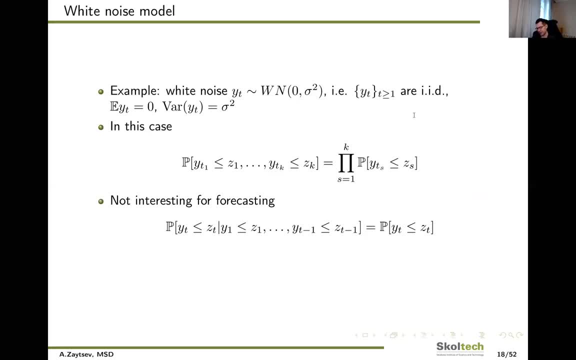 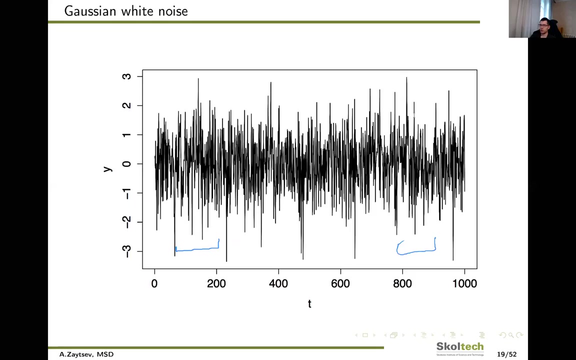 we can say that, okay, if all variables are independent, then this probability equals to this probability. it doesn't depend on our previous values because all random variables are independent. so we can't do anything interesting about forecasting. maybe in very specific cases can be useful, but in general it almost useless model. let's just say that we don't have any dependence. 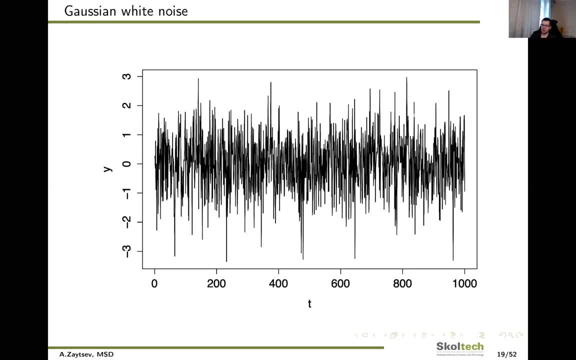 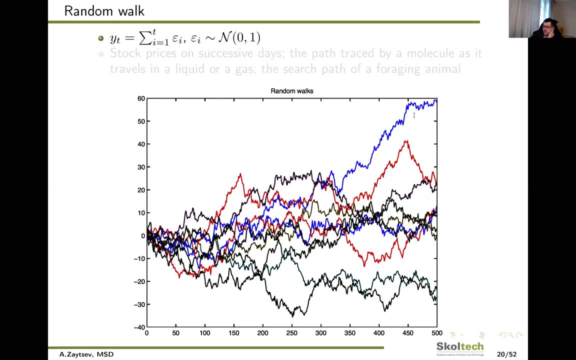 and actually we can look at this time series as a number of separate events. not very inspiring example, but, i suppose, pretty simple. here, for sure, we can try to make the model more complex and we, for example, can use the random walk paradigm here. the random walk model and what? 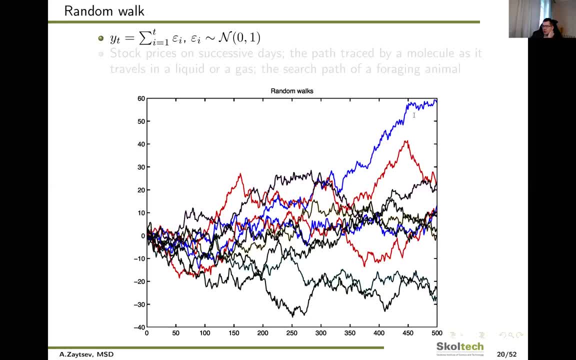 this model is about. in this case, we say that each observed value is sum of a kind of large number of different noise values. in particular, we can say that for each epsilon we have observations of it, and y is the sum of epsilon at each time step is. each epsilon is generated from some gaussian distribution with specified 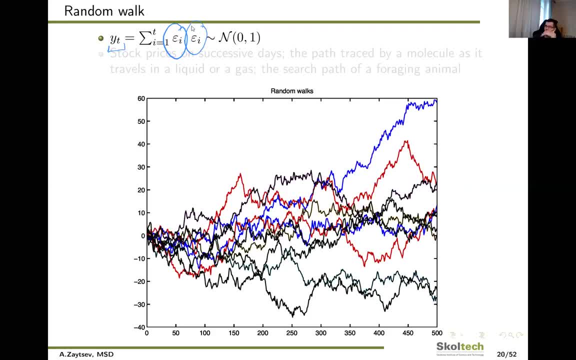 a mean value and specified noise also, not that this kind of usage of white noise model, but in a more clever way, because right now we can say that this absence, actually the series of all epsilon here, is white noise. but if we sum these values, then we no longer observe white noise. instead we observe the quite 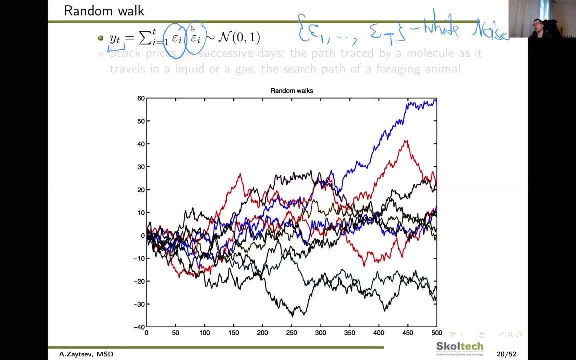 interesting and quite realistic dependence of each pair of yt and some past value of it, minus one, for example, and we can say that in many applications these are quite reasonable assumptions. to have this random walk time series model, for example, it can be stock prices on successive days. 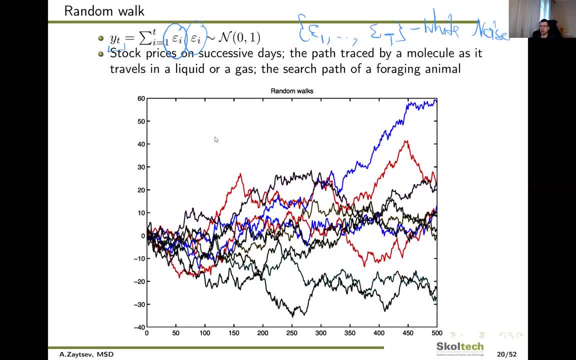 when we observe a molecule that goes through a gas or a liquid, or we see that we have an animal that travels through like a forest and searches for a prey and so on. and all those cases is a reasonable model, don't have much parameters and so on. so let's try to. 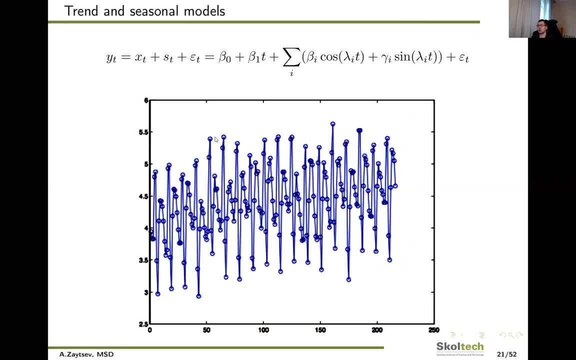 imagine something different we can try to use as transient season models- as we already know that this is can be crucial- or to have correct trend model and correct season model, and so we can say that, for example, our trend would be some linear function, as we expected before our seasonal. 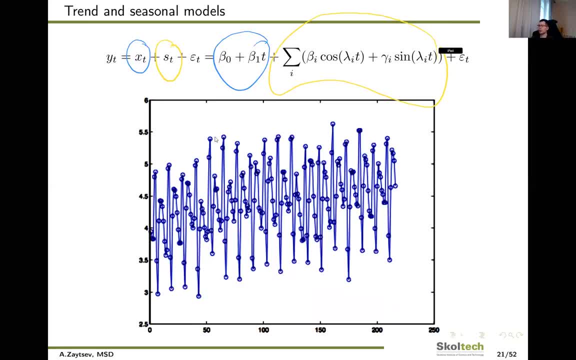 component is something identified by harmonics for cosine and sine function and for the noise. we can't here introduce any interesting one, or we just say: nice, it's just nice, let's don't talk about it too much. and after the composition of like this, so the composition of our time series to seasonal model and to a trend we are ready to. 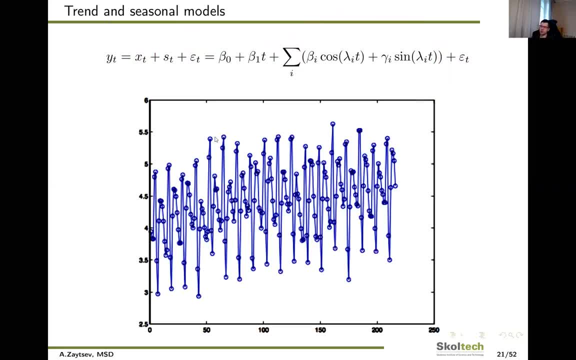 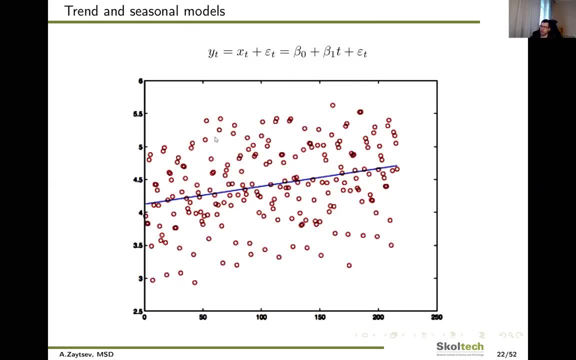 provide some description of our time series model like this, so we can use the time series model to our time series model and to attend. we are ready to provide some description of our time series model and also some, even some, predictions. so for data we have, I don't know what this particular data. 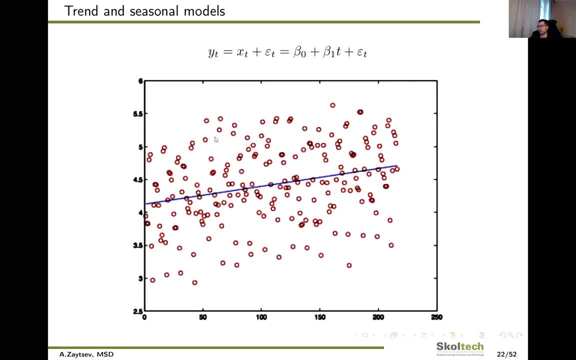 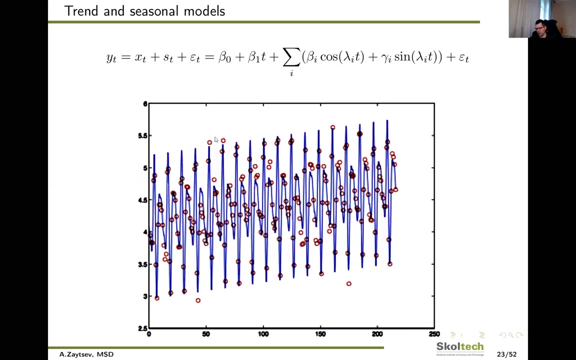 is about, but it doesn't matter too much. we have this linear model here like this, and it's pretty easy to see that we can do it and we can try to to make it work, even for this pretty noisy data. also, we can try to go one step further and estimate parameters for. 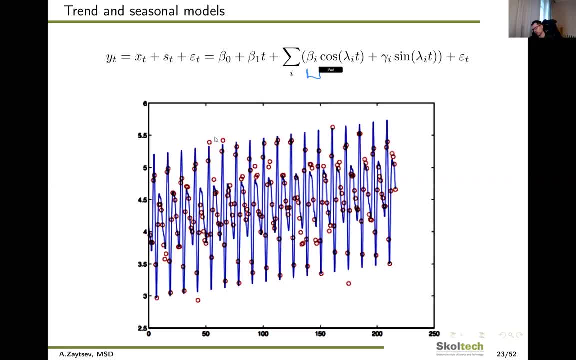 this guys on periodicity. so this is a efficiency estimate. also we can try to select a lambda, so the period of the time series, in a uniform value. using some expert knowledge also we can try to optimize it. but I suppose it is assumption that this it's not. definitely lens this 벜aOOc y são surtout nós vamos所以呢, um tem uma ideia do objeto é previsores, são o um ponto noir dse uhar o que ele puis um tempo em que um dist complications, but I suppose it's this is something that is, it's not. standardizing. it's notеры úрон um controle em que é untuk um beautiful. it's an example, general-ivel, quando we measure in the bright need to tell more, in bestimmę, try to optimize it, but I suppose it's a Xue, is something that is. it's not. 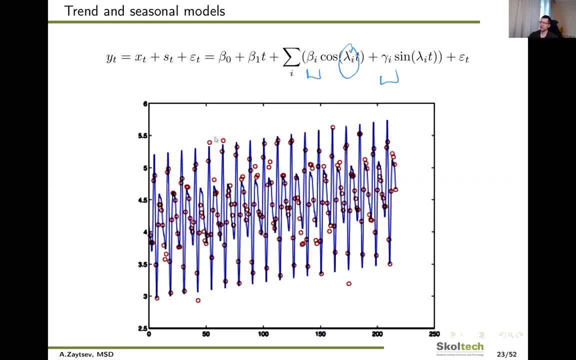 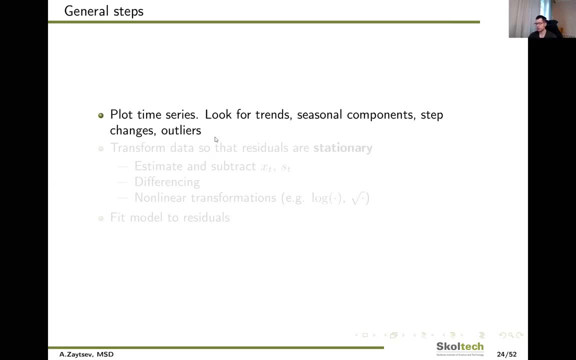 a very good optimization problem and i suppose it's a very rare case when we try to address this lambdas to make the time series better, so no one does it. so, to sum up, we tried to introduce some models for each part of our training data, and we actually do it like this. 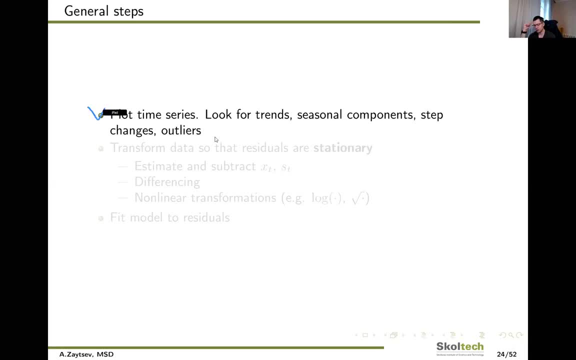 we started with potent of time series and looking for some components that are vital to the model of time series in general. trends, seasonal components, changes like abrupt one. when we like observe, one can see this up and we have another one, and so it is, and we should somehow reflect it. 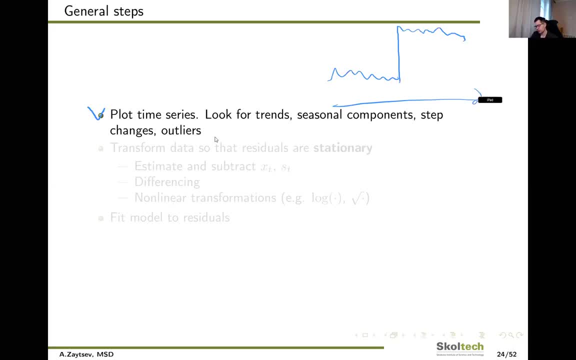 when we are working with time series like this. there can be other examples here. for example, we can have outlier here, here, here and here, and we also should include this knowledge about the model, because otherwise it would be quite risky to make any reasonable assumption and any reasonable time series models. because of the limitation, because we 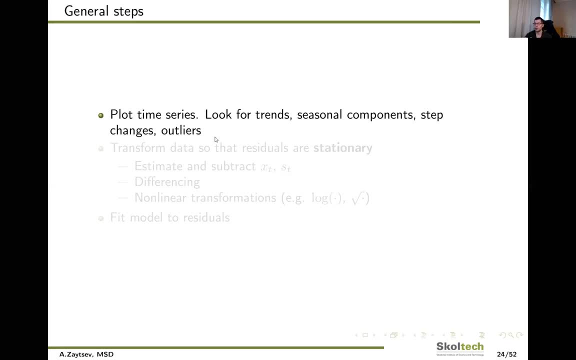 wanted these models to be as simple as possible, at the cost that we don't make them like bad. so they fit to the data quite well, and so, after plotting time series, looking at it, analyzing it with an expert, usually we start with transforming the data to make it stationary, and this what we talk about. 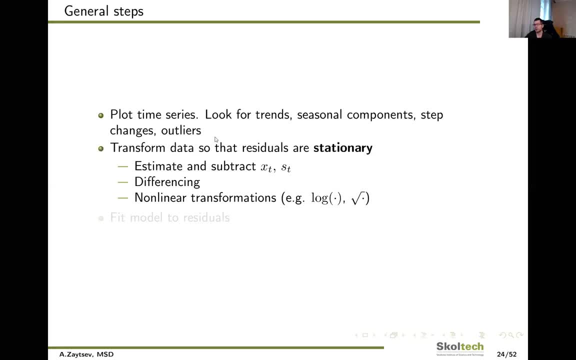 later. why is so important from theoretical point of view and also from practice too? i saw we estimate a substract trend and seasonality. uh, another useful trick is differentiating. so i suppose we have time series like y1 and yt capital. uh, then we can try to look at something like: 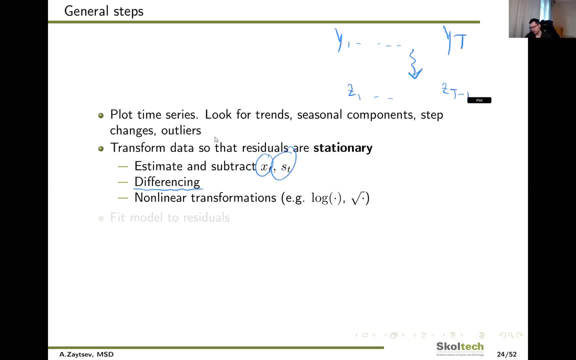 that one is that g minus one and each z is one step difference. that she is that g plus one minus t, and in these cases we have to look at something like this and we can see that it's pretty easy to model it like this. also, it's useful to have some non-linear transformations, if you observe that we have. 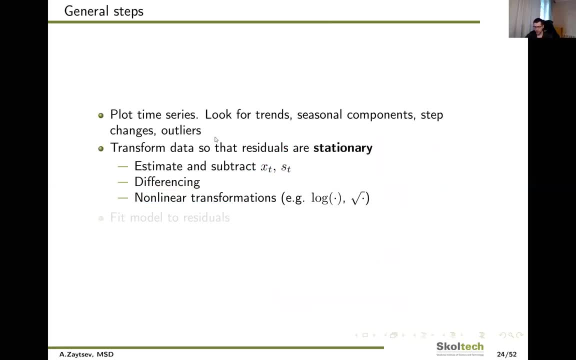 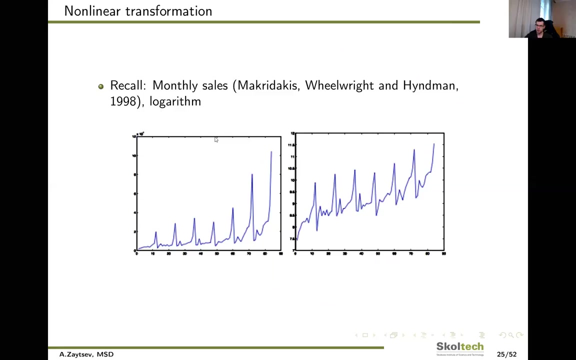 exponential trend and we want to make it look smarter and better. and also, what's crucial, what's worries us a lot is that if we identify the model now, we can fit the model to residuals to make it look better and some it. let's provide another example of what we 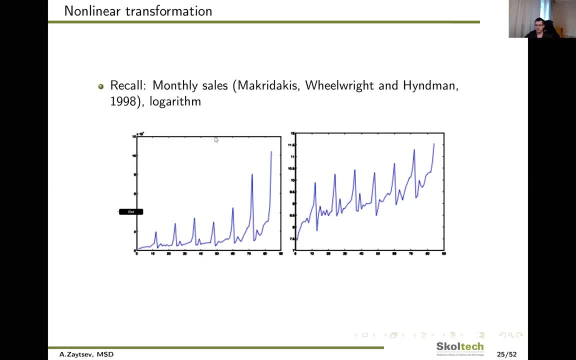 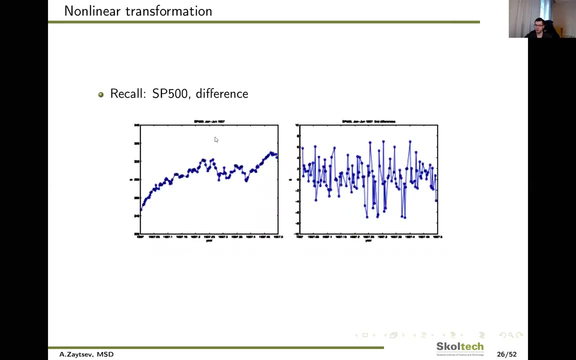 what we do here, and so we have this modular sales data and, as you can imagine, it's pretty important to have this logarithm scale here, and after this we can work. another important part of the processing of time series data is taking the difference between neighborhood values, so here we observe some trend after. 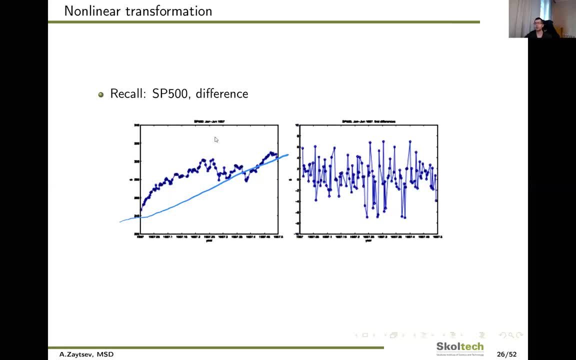 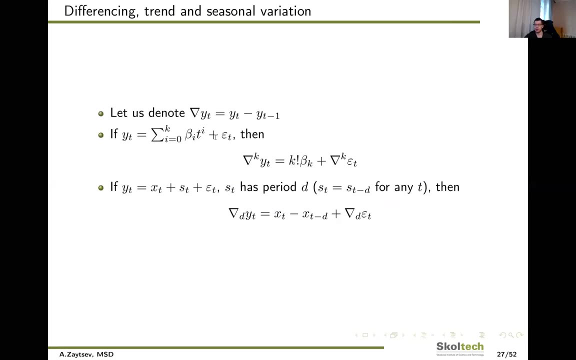 differentiation, we observe almost north trend. it's pretty easy to model something like this when we are talking about the data itself. what else we can do as tricks? we can try to make it look better and make it look more reasonable and more useful, and this is like: 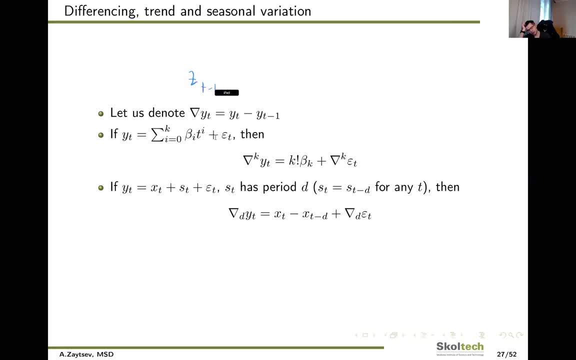 what i had before as a t minus one. we can designate as delta yt the difference between the current value and the previous value, kind of estimate of a derivative, you can say, and so on. and for a particular reasonable time series models we can observe what this difference is and how it's related to. 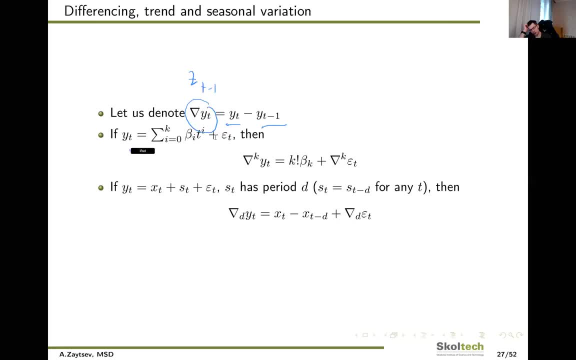 uh, these difference variations for, for example, for yt, that has this polynomial structure, polynomial model, so each time t we have this t plus one, and so on. uh, then we have the model like this for the difference of keys, order for our guy y, and also we can try to imagine on what's going on for another example of more. 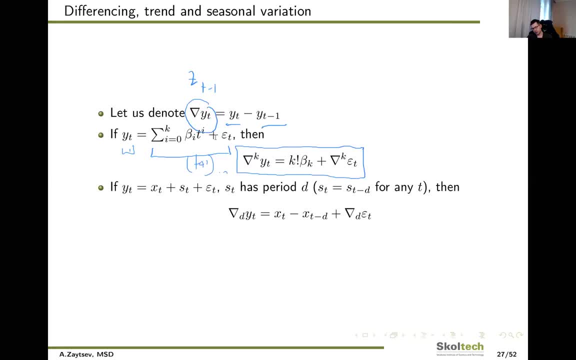 classic decomposition, to the trend, to the seasonality and to the noise, where s3 have the period t and we observe the difference between the value here and in these steps, so it's like yt plus d or yt and yt plus d. then this difference has for sure the form t minus d, i'm sorry, and t here. 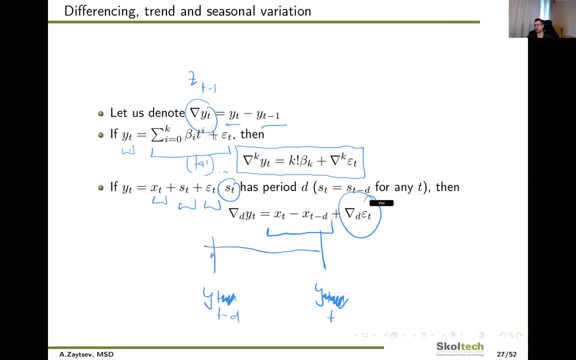 like this, and also, if the noise is not id, we add this difference for noise and as the value of st equals to the value of st minus d, then when we are doing the subtraction, it cancels and we no longer have. this is my component, this, why the reasons? one of the reasons: why do we even need this kind of behavior? so? 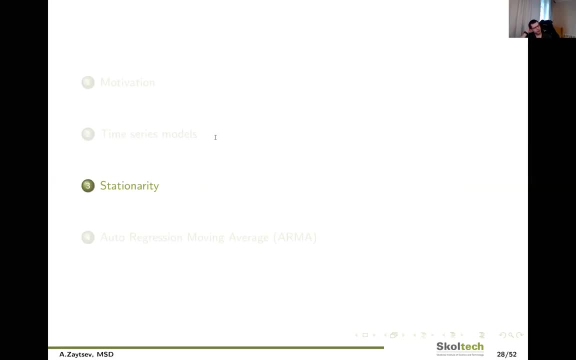 we looked at some models and provided some useful examples on how this model behave, and now we are ready to go to the next part and, in more details, discuss the stationarity of the data and what the does it mean. the most strict definition is strictly stationary time series and it holds if 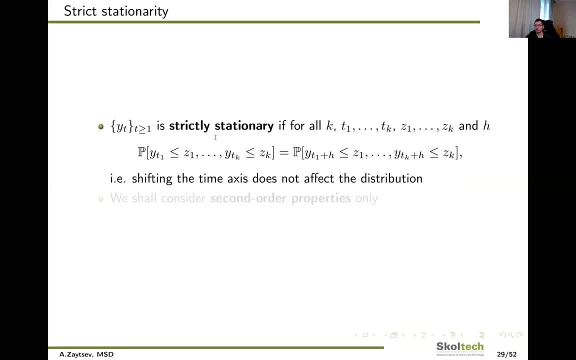 for all value of keys and for value of time series and for all letters. we can have the decomposition like this if we shift to okay from the present to something like present plus h. so time series like this and time series like this of the same length- there's a joint distribution, is the same. 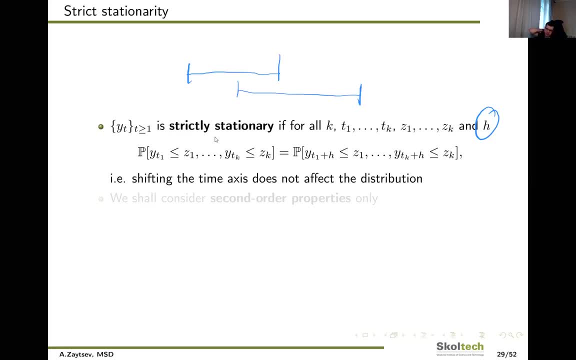 and we don't have. no, we have no change here in the distribution, uh, but it's quite hard to check. do we have the same distribution? so instead to use a simpler model for stationarity, we will consider only first and second order properties here. so suppose we have. 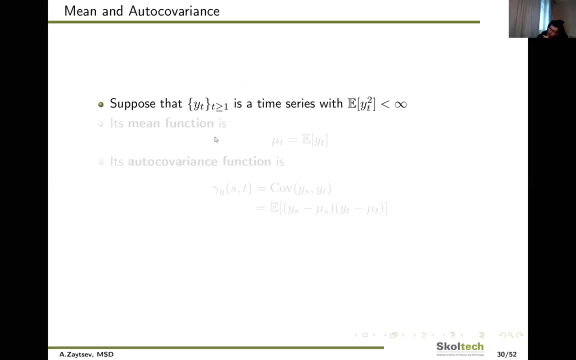 a time series and expectation for each, at each time moment is smaller than the infinity for the square of the y. and also we have some mean function and some after covariance function here. uh, for mean value. okay, we suppose that we have some mean value related to each particular development and we have some after. 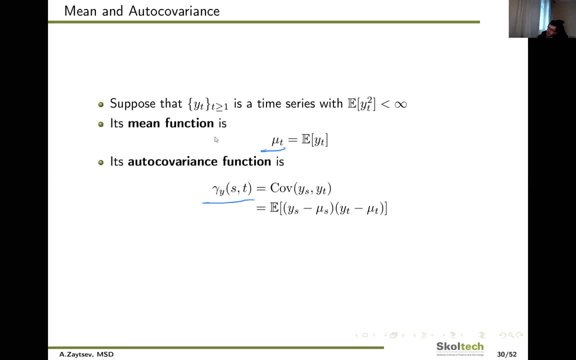 covariance function related to two selected moments of t. it can be okay. here is: it is a covariance that is defined as expectation of y minus no related no and y t minus t related to it, and so we can say that y is equally stationary if mu, the first moment, is independent of t. 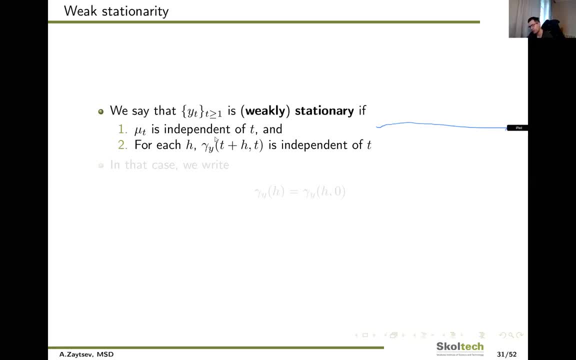 so we have the same mean value- uh, doing all the time series- and also the difference between. okay, the covariance function is also independent of t when we shift to it, so it can. the same function depends only on the difference between t plus h and t depends only on ash. 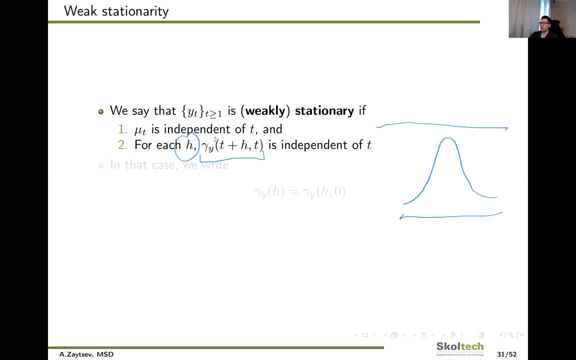 for us it's particular number. in this case we can, for example, replace this: more complex designations when we have two guys, two terms, action zero to the case when we have only one term are related. only okay to this time difference ash here. so we are pretty happy about it. 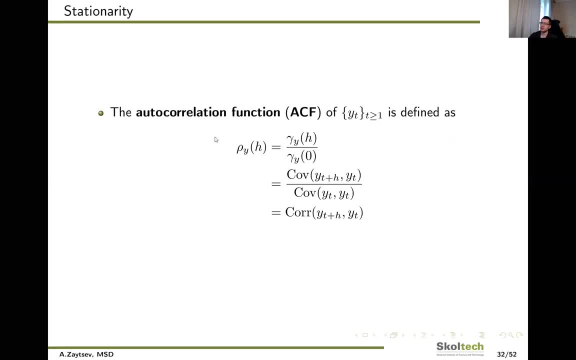 and we can go further and say that we are interested in after correlation function, and the after correct function equals to the ratio of the correlation function for the difference ash divided by the after correlation correlation function for the difference zero. and in this case we say: this is the correlation and we are interested in particular. 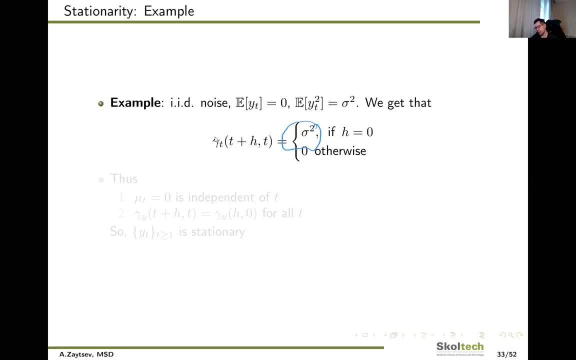 correlation. let's see if the examples we discussed earlier are stationary or not. we start with identical distributed independent noise and we can see that the correlation function is equal to zero and the variance is equal to sigma squared. in this case it's pretty obvious that mu t equals to the constant and also we can look. 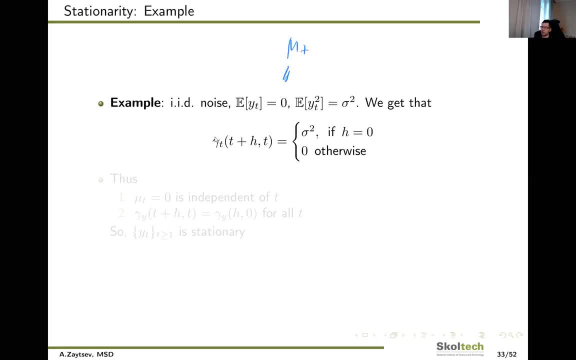 at the correlation function, as a correlation function has, like sigma, squared value if h equals to zero and zero otherwise. this is pretty much expected for the correlation function for different contentMPyst. this is what we're looking at. okay, let's take a look at this. doesn't like me. 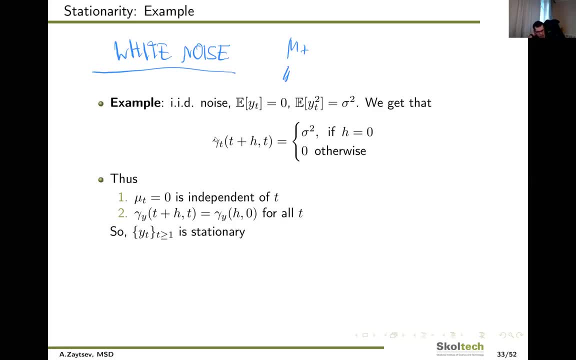 there weren't any additional contrasting characteristics here of different types of sound effects or class. maybe we can try toétique one, two, two, three. oh, they are almost the same. the difference again is so far in of my current model what we can personally do with basic stationarity- weak one for this particular model, so it's very easy to check that. 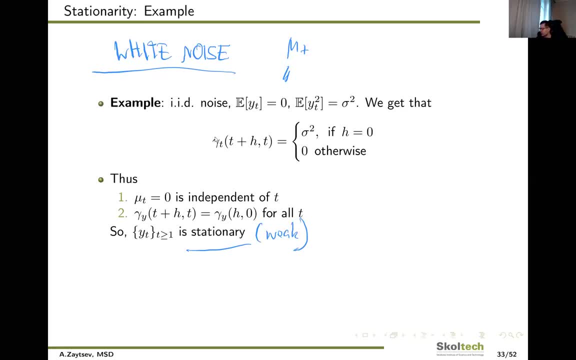 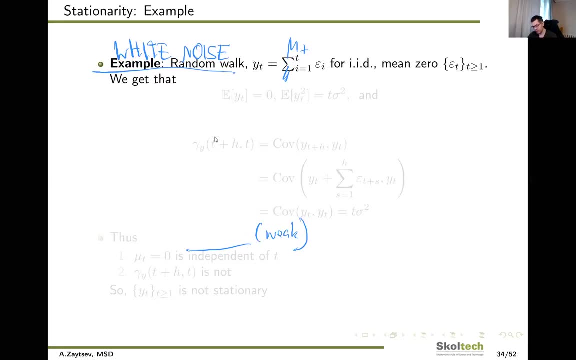 okay, i suppose white noise has almost all nice properties we would like to have for time series. the only problem is too simple to model something useful. let's have another example and check if the random box follows this assumption about the stationarity or for our particular case, we can. 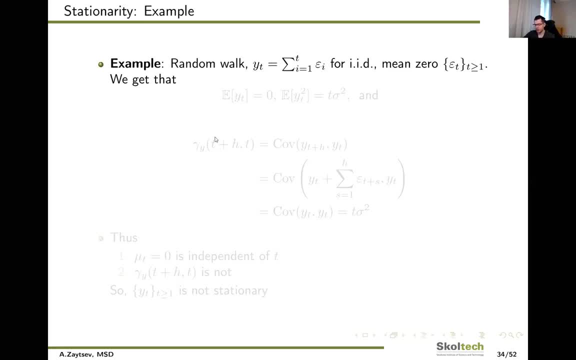 consider this stationarity. we say that our y is sum of independent epsilons, and each epsilon actually is a part of a realization of a white noise, and so we say that our mean value is zero. and also we can now say something about the variance, as these guys are independent. variance of sum of independence, random variables. 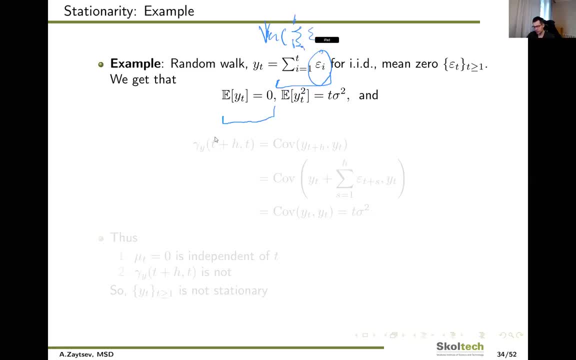 equals to the sum of variances of this independent guys and, as a result, we have the variance that equals to g times sigma squares, sigma squared, because each epsilon has this form. okay, let's calculate the mean value and covariance function from here. we already have zero, so it's pretty easy to calculate it. 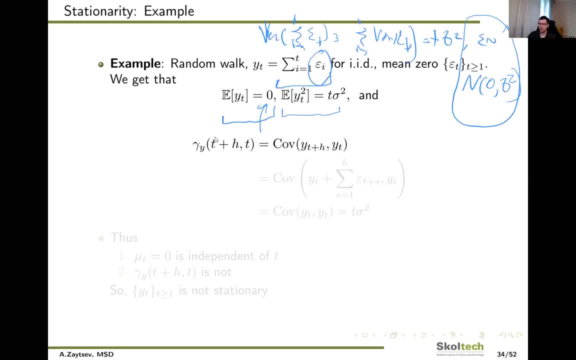 uh, for the covariance it's a bit different. we say that this guy, the covariance between yt plus h and yt equals to this covariance. so this is what we already have and this is an addition we have for, because of this, additional terms later: from t to t plus mdt, and so 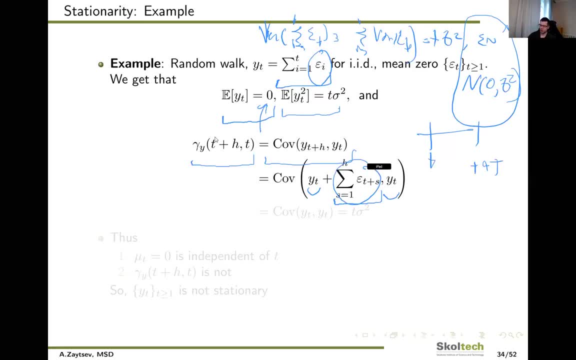 these guys are independent of yt, so we don't care about them. what's less equivariance between yt and and y t? okay, the same two variants: g times sigma squared, so mu t equals to zero and it is independent of t. gamma is not, because it depends on t, not only on us. so you can say that this is. 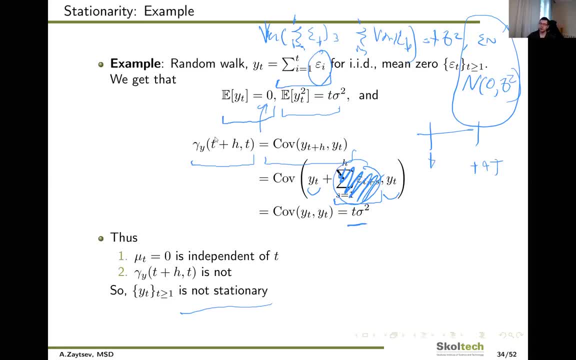 fixed sonarity does not hold for random walk. so we okay, we can try to make it stationary and consider not wise but epsilon instead, and we go back to the case of white noise. so after normalization we can go back to the length of stationarity, but for this particular case, simple. 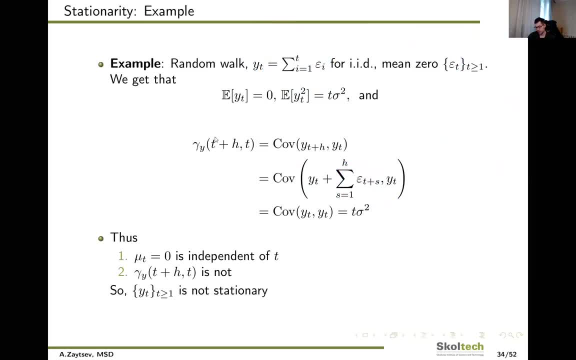 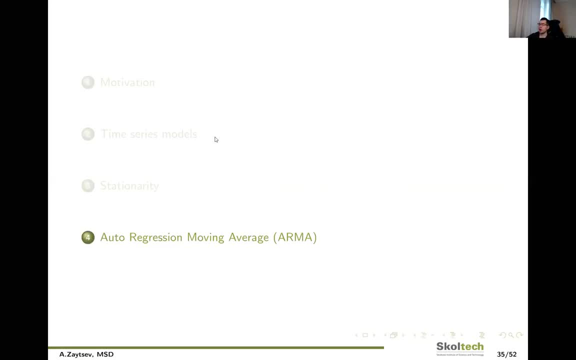 check shows that this time series is not stationary. okay, let's look at one of the most popular models in time series: modeling after regression and moving average. to conclude the lecture we have right now, we start with a simple but quite effective model for a time series. it moving average, or moving average one process, because we have only one. 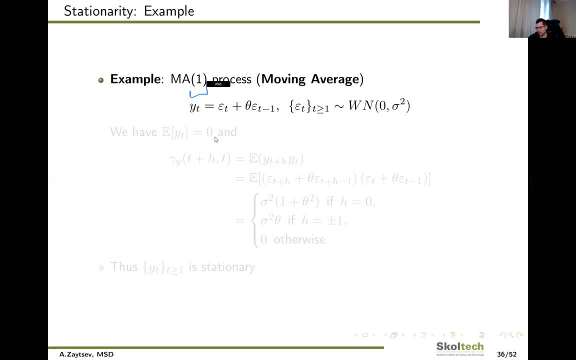 component here and it equals to the sum of the noise here plus noise as a previous step times theta. as each epsilon is a part of a white noise process, we can evaluate the mean values. that equals to zero and also we can try to evaluate gamma, and for gamma we write it as: 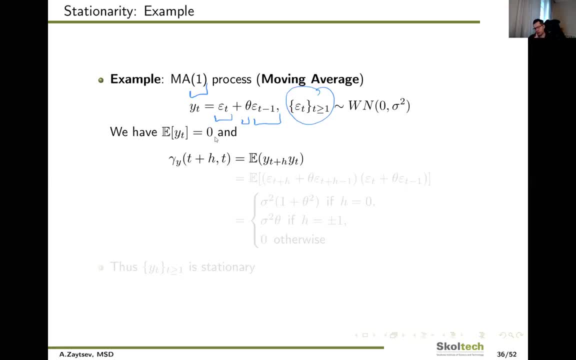 the expectation of these guys, because the mean value equals to zero, and so it's like this, and also, as epsons are independent of each other, we have three possible cases: either h equals to zero, then we have this guy for sure, because we have sum of two independent variables for each of y. 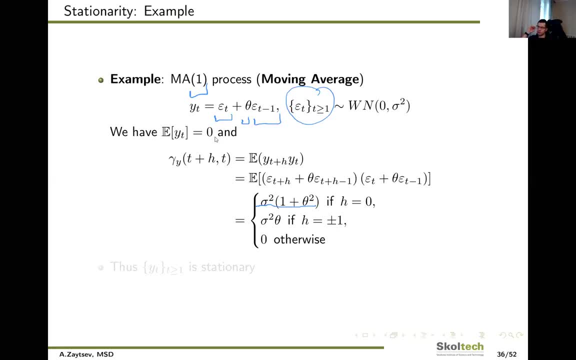 and they're actually the same independent random variables. if actually equals to plus one or minus one, we have this intersection, but with a coefficient teta, and so we have the variance that equals to this guy. otherwise, these two random variables are too far away from each other, so it equals to zero. so, as you can see, 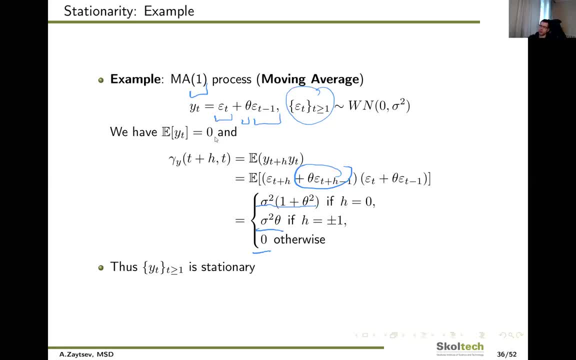 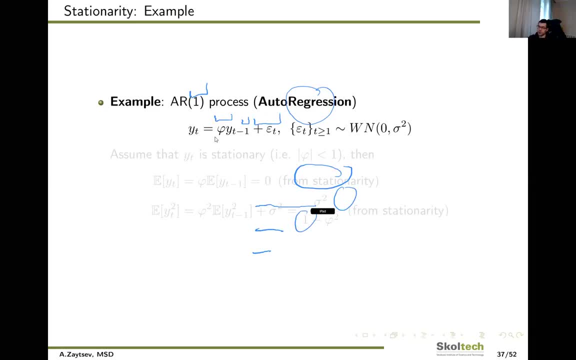 mu doesn't depend on time. gamma also doesn't depend on time, only on ash here. so we have stationary time series. another interesting process we often talk about- it's pretty natural way to think about time series- is: after regression: uh, it's about that. the next value is a previous. 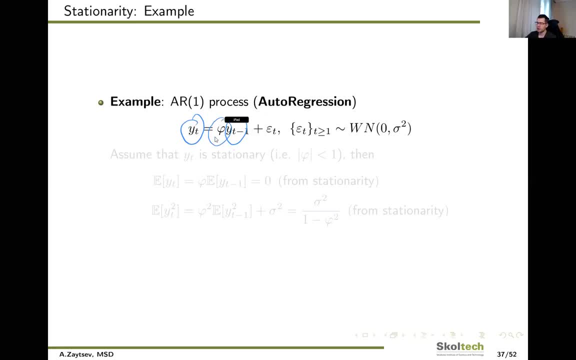 value times, some phi plus noise. as usual. we assume that this noise is a white noise. with gaussian random variable of zero mean and sigma squared variance. if phi is smaller, phi is smaller than one, then it's kind of conditions that this time series is stationary. but also we can try to identify the mean values. that equals to zero again, and also. 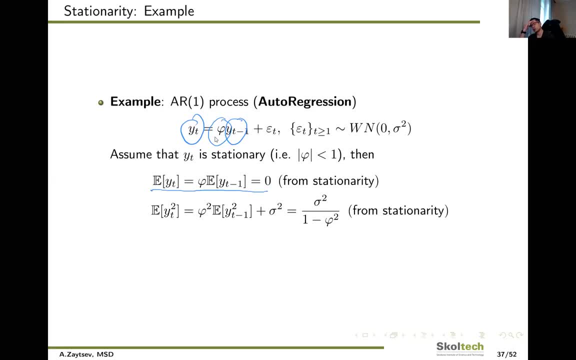 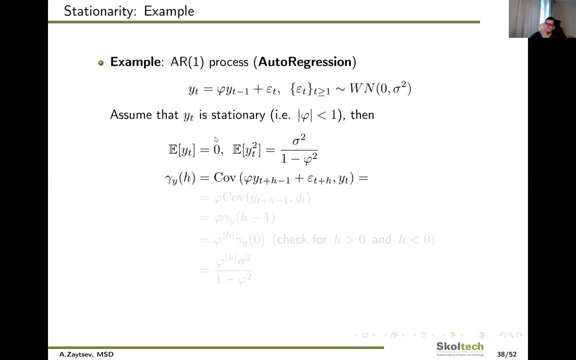 we assume that for for u, for sin Q, so so it sigma squared equals to x 1 minus phi, phi squared, and so we have the formula like this for this mean value and so on. also we can try to calculate gammas if we assume that we have stationarity, and so 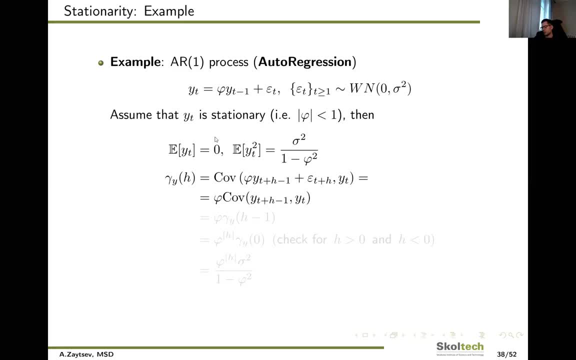 on. we can write y in this way. then this is like this: because this white noise that isn't related to y, so we can put phi outside of covariance, and so we can say that each time we increase step by one, we multiply the value of gamma by phi, and so it's like this: 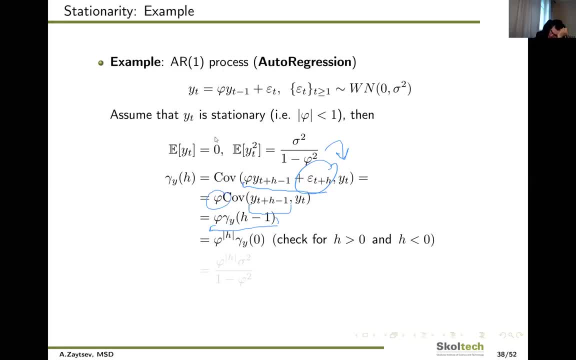 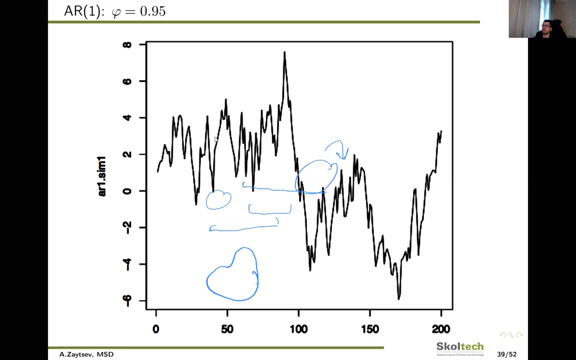 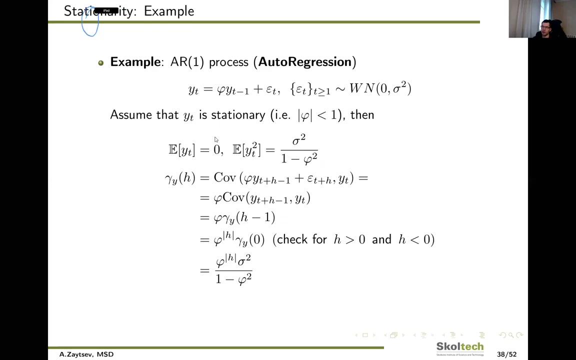 for each value of h and if we substitute- oh i'm sorry- gamma y of zero, then we have this formula for gammas and we can look, for example, at some of the regression process of the first order. first order means that we have only one term here. we don't have terms like phi 2 by t. 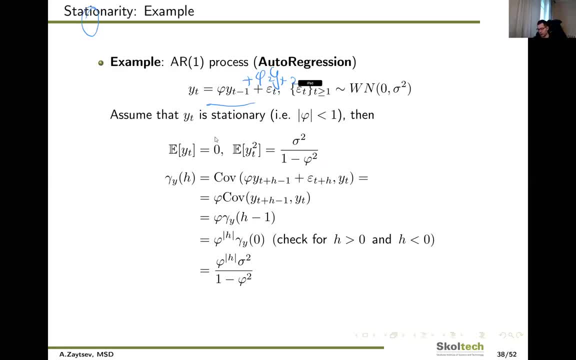 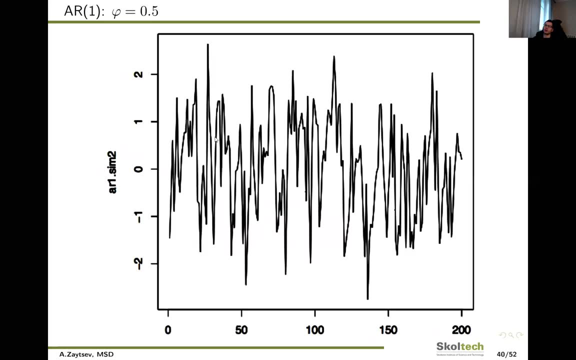 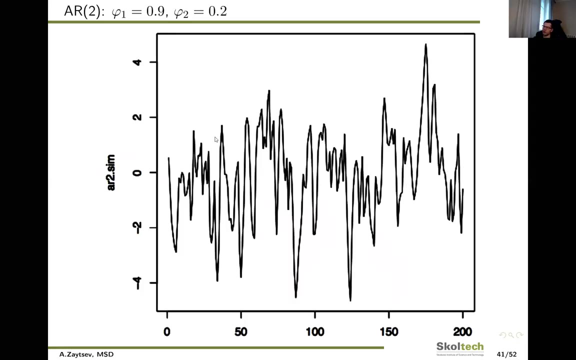 minus 2 and so on, the first term after regression, and it's like this we can increase phi. if you have our decreased file, i'm sorry, we would be closer to white noise if you have large variance for this white noise, sure, also we can try to have more components here. 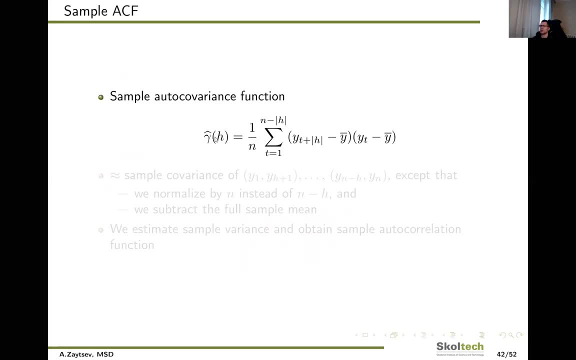 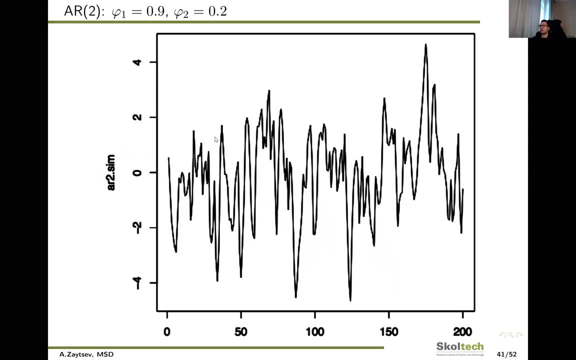 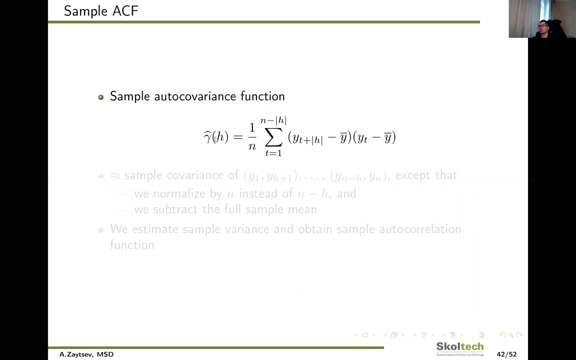 and it's kind of smoother and we can prove it later, and so So we have another examples of two popular stationary time series models And also, to conclude, we have a nice tool to identify how stationary the time series is. We can calculate this after covariance function using the sample we have and what we can say. 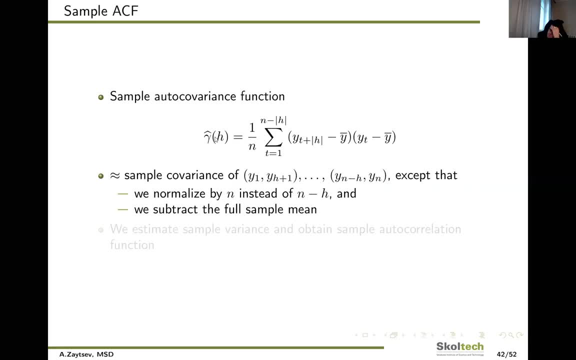 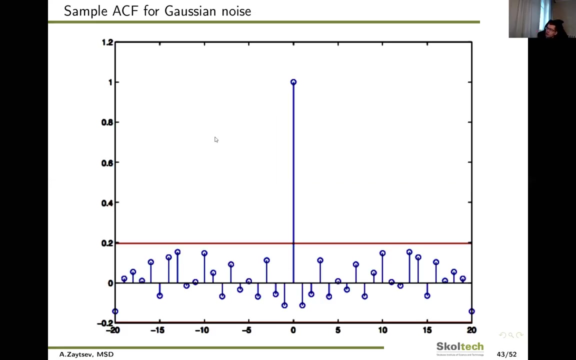 it's like this And it equals to the after covariance that we calculate from the data we have. So we have sample variance and sample after correlation function. that can look at it for some popular models we already discussed today For white noise. you can see that this component is large. 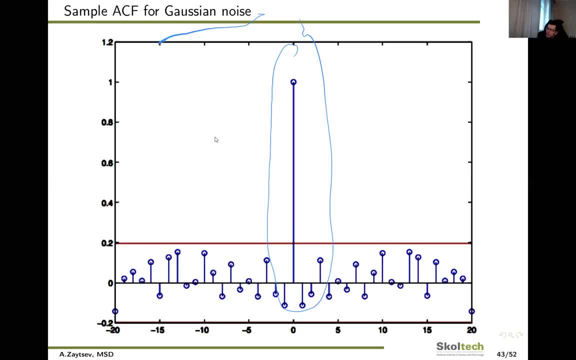 But all other components are small enough And actually this value behind this hypothesis testing bar for that. if the correlation is more than 0.2, then it's not significant And what we can see that we can do, identify only one thing from component related to zero. 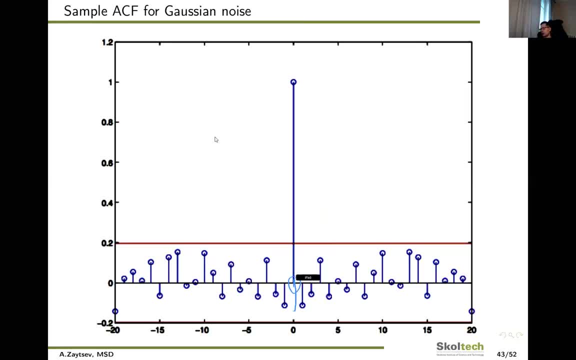 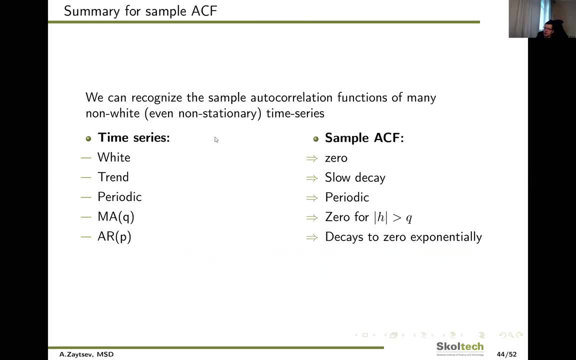 related to the time series itself. that is kind of correspond to lambda squared. If we try to do the same thing for other after correlation function for other processing, we can say that for trend we have slow descent of sample after correlation function for 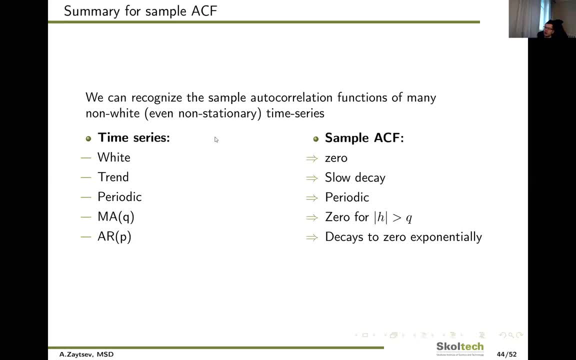 periodic time series. we have periodic after correlation function for moving average and after regression we have a bit different station. For moving average it equals to zero. Our time window is larger than the order of moving average. For after regression we have exponential decrease of the after correlation function. 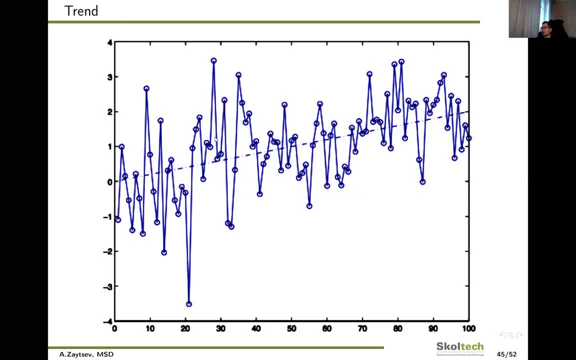 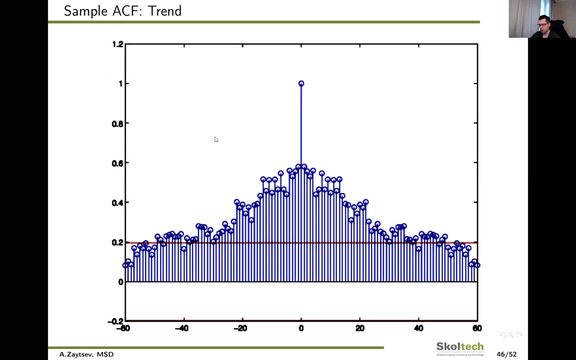 to zero if we increase the h here, And it's pretty easy to see from the plots, But it's easy to imagine that we should have something like this If we have a simple linear trend plus some noise And a correlation is like this: okay, what we would expect. 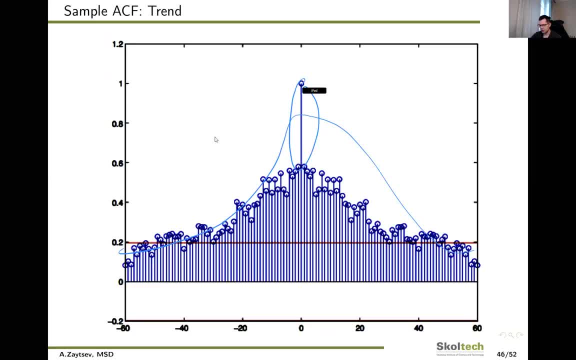 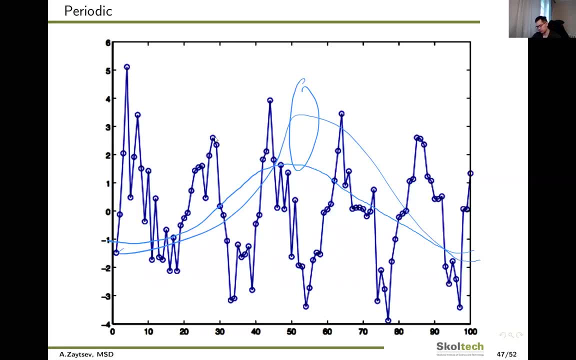 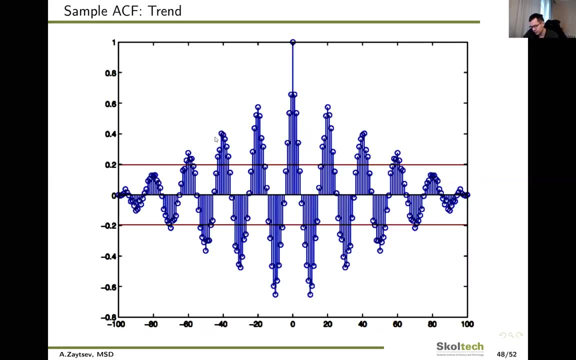 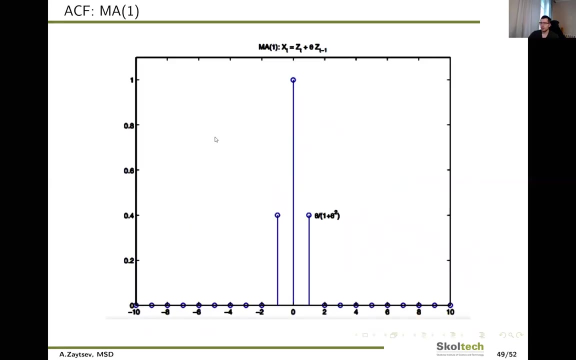 Also, we have this difference to like trend after correlation function because of we have noise here. If we have periodic time series, we also can observe that right now we have this periodic high variance of covariance function here For moving average. It's pretty easy to calculate it like this: 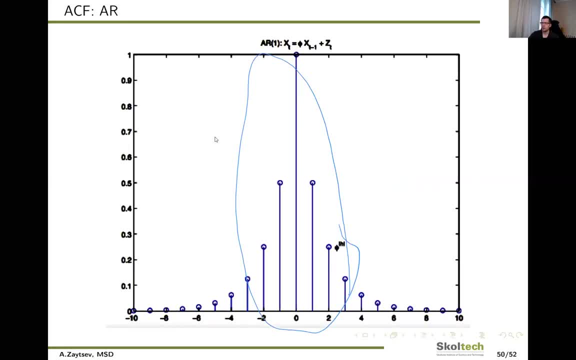 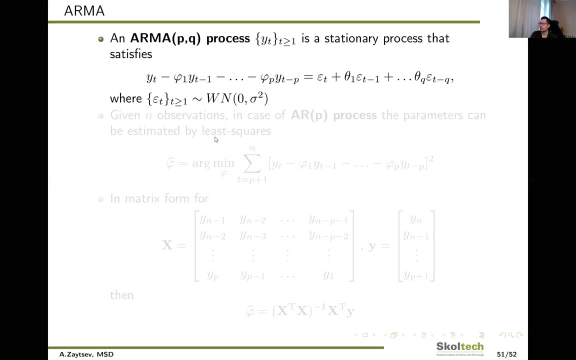 So we have only small number of non-zero components. After regression, as I told you a couple of slides before, it has an exponential decrease here, Finally, we can try to generalize what we have for moving average and after regression and the order of these two processes related to the number of steps that are applied to. 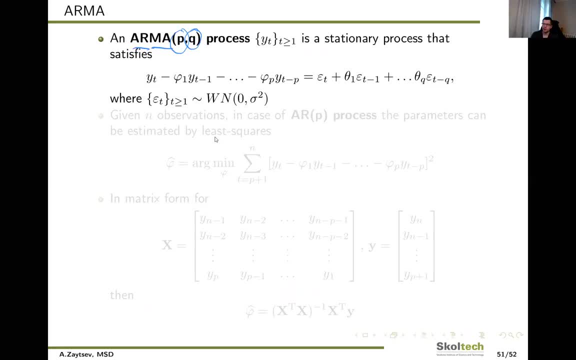 the process. Okay, After regression. new component depends on from the past And that is related to moving average: cast steps one side, cast steps other side. And so we can say that if our time series is stationary process and if it's arm arm, 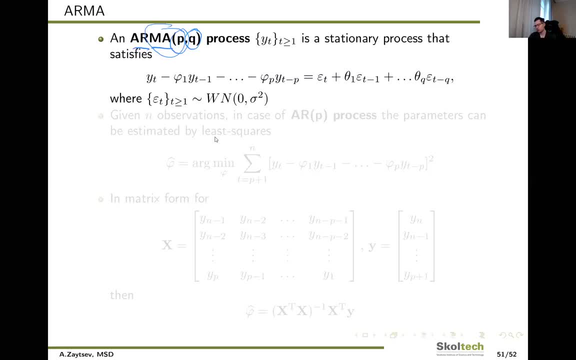 process. then we have the decomposition, like this For our Yeah, Now we have the displacement, We have the displacement and we have the rotation here, And so we can do the same thing to the next unit For this unit, And we can see that the resistance is the area of this component. 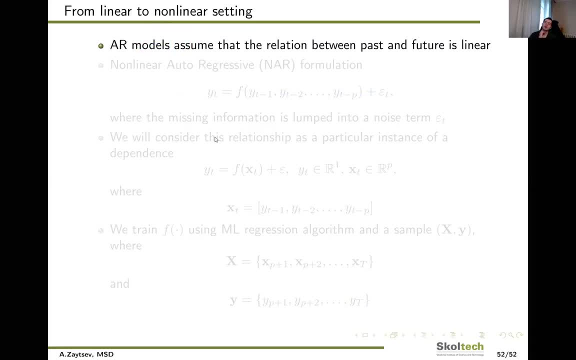 So we can say that the resistance is this area, But the non-zero component is also linear. We can interpret: the〔fficacy〕 is the area of the component that can model. many common relations are between time series. we can try to use it in a different. 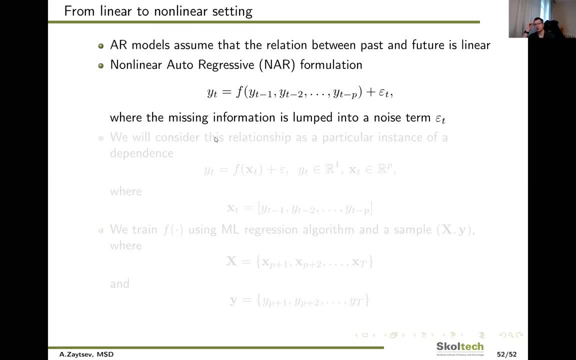 way and use a linear model for it, and this is we are going closer to the word of machine learning, because we don't know the true dependence between yt and previous various of ways and and so we can try to train f in a very common way. everyone of you, i suppose, was doing. 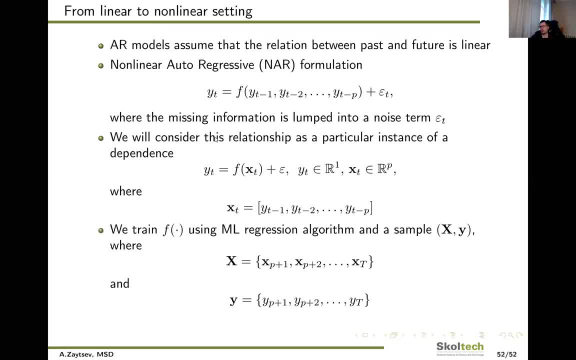 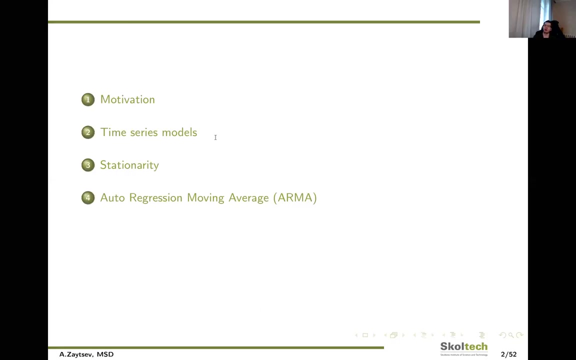 long times but in the end we have variant approach and solve it. but now we can try to do some in a non-linear setting. but okay, we can see if it's a good idea or not for everyone particular case. so what we actually did: we give an overview of classic models and classic assumptions. 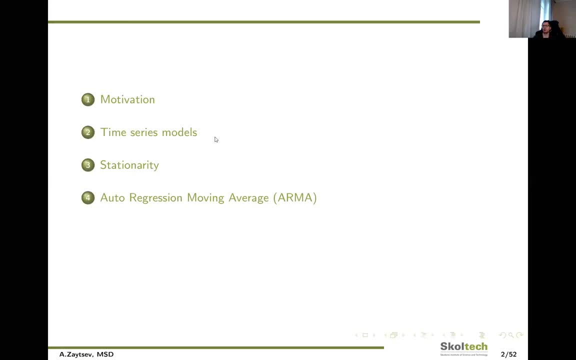 and how to check them for time series models. we understand that this, quite understand, understood that this question is very important and, in a simple terms, we can try to have quite complex models and for this model we even. they are quite simple. you can do a check for stationarity and 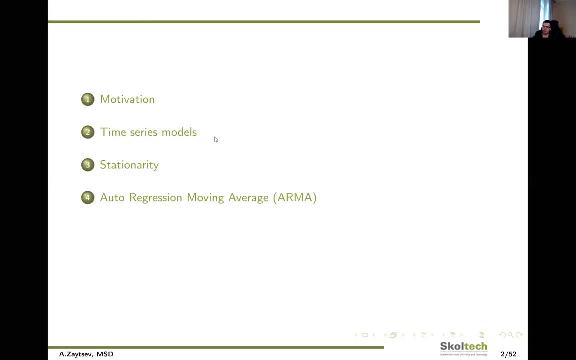 kind of use more complex models. that's kind of union of the models we have before after regression, and moving average model in my opinion is kind like a linear regression but is more specific to time series we are working with right now. thank you for the attention and i hope you're enjoying. 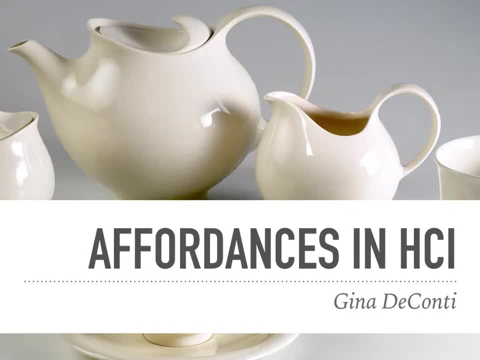 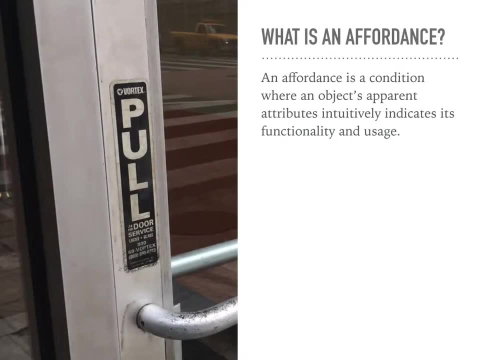 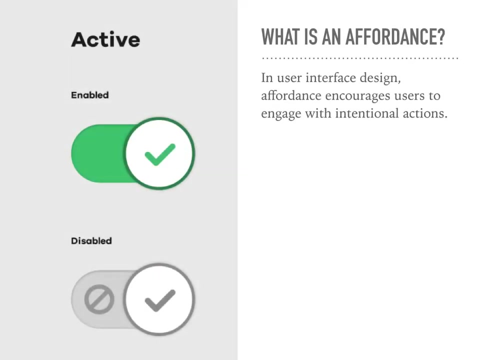 Affordances. in HCI, An affordance is a condition where an object's apparent attributes intuitively indicate its functionality and usage. An affordance is a pleasing quality of a user interface which organically guides people to accomplish their goals. Affordance when employed as a tool. 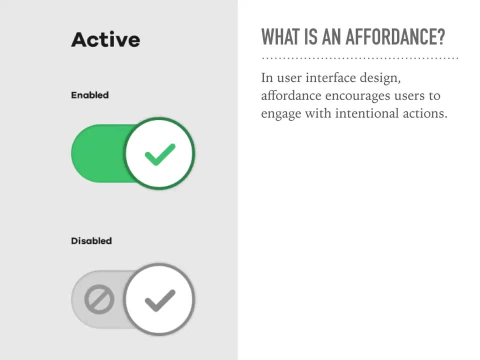 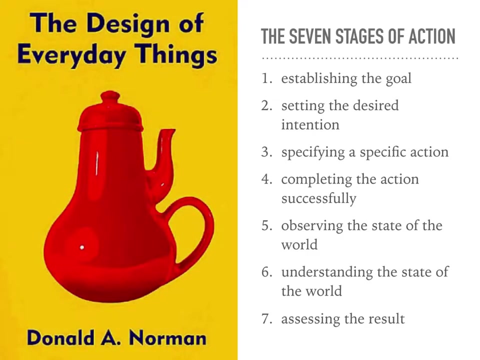 makes the designs more natural to use and encourages users to engage with intentional actions. Effective affordances result in higher conversion rates and other beneficial outcomes for users. Donald Norman, in his book The Psychology of Everyday Things, advocates that designers use the seven stages of action as an aid in creative prototyping. The seven stages of action.